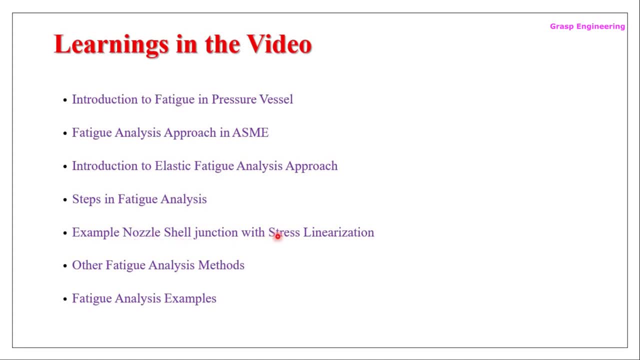 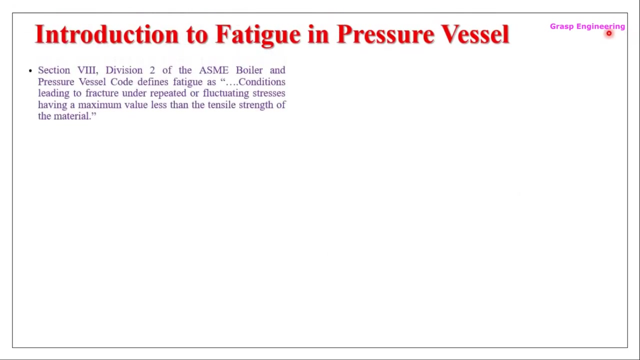 And we will also discuss about the example of nozzle shell junction, along with stress linearization and how it is correlated with the fatigue analysis. And then we will discuss about other fatigue analysis methods and we will discuss later on or at last, fatigue analysis examples. So this slide represents the introduction to fatigue in case of pressure vessels. 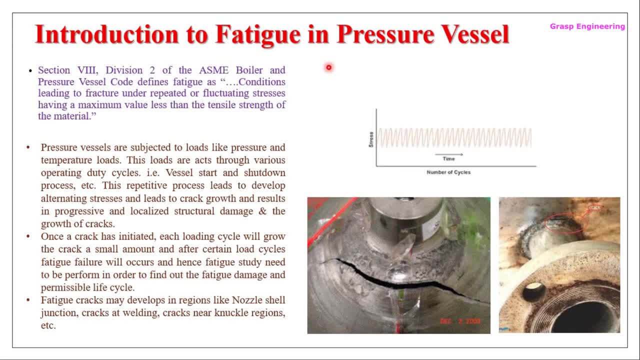 So we will discuss about the example of nozzle shell junction, along with stress linearization and how it is correlated with the fatigue analysis. So when we talk about pressure vessels, there are different number of codes are developed across the universe. The most widely ASME boiler and pressure vessel codes are used by the pressure vessel manufacturer as well as pressure vessel service providers. 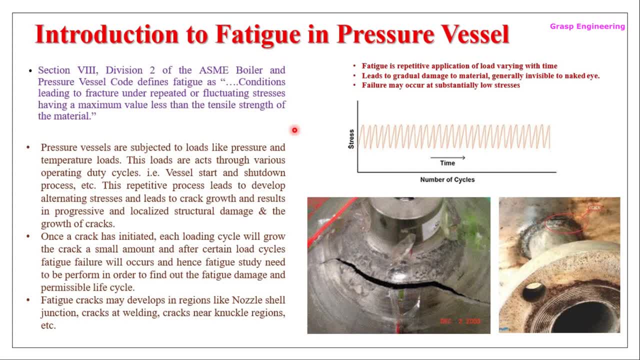 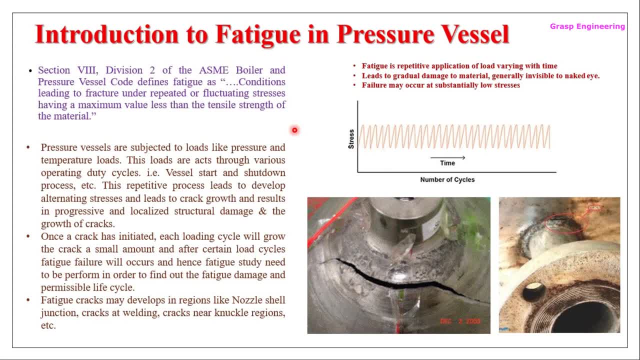 So it is basically American Society of Mechanical Engineers which develops this boiler and pressure vessel codes, As well as fatigue analysis by elastic approach in this video. So, as per section 8, division 2 of ASME boiler and pressure vessel codes defines fatigue as a condition leading to fracture under repetitive or fluctuating stresses. have a maximum value less than the strength, size, strength of the material. 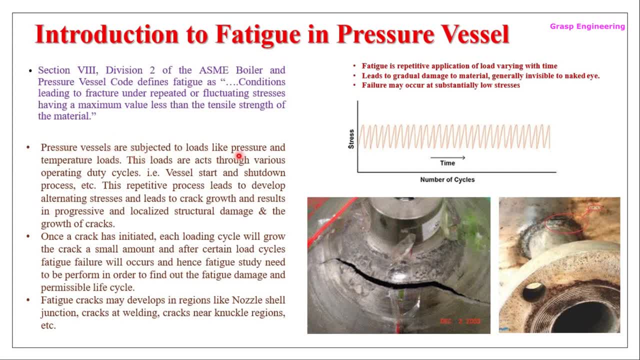 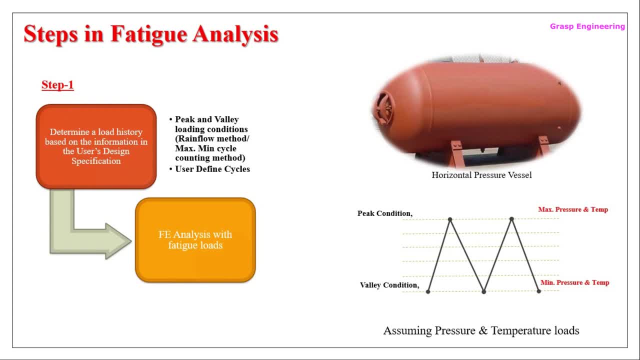 well as pressure vessel service providers. so what does it mean? so, if you see, here, as we know that this is one of the example of horizontal pressure vessels and we know that there will be a pressure or temperature loads, so here we need to first find out which is the valley condition. so valley is nothing. 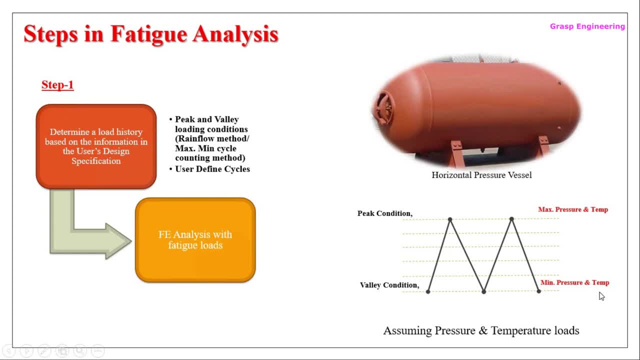 but your minimum pressure and temperature. where the loads are, you can say the zero or minimum loads are present and peak is nothing but your maximum pressure or temperature. so peak is nothing but your condition, where you will find the higher loads. so the very first we need to identify the peak and 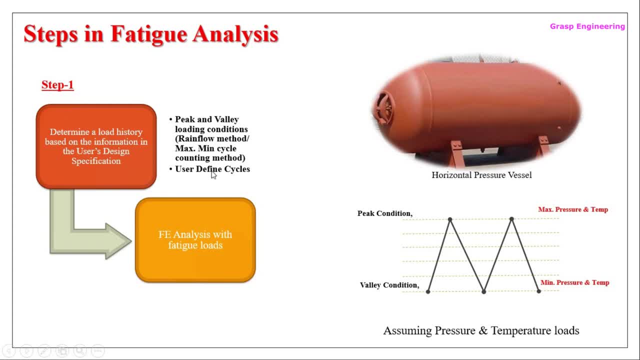 valley conditions. so this can be done by rain flow method or maximum and minimum cycle counting method or also by using user-defined. so when you refer any pressure vessel sketch you will find on bill of material. there are few manufacturers which can define what is the maximum uh your pressure, as well as what is the minimum pressure. 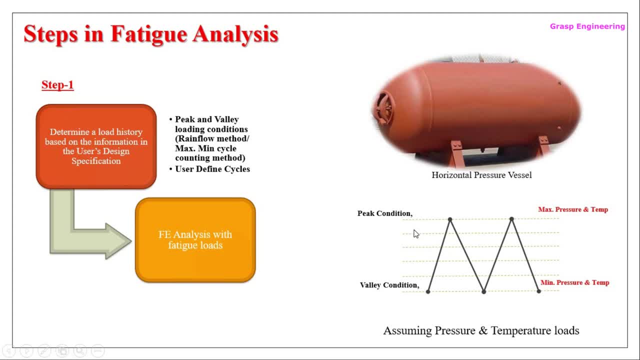 so based on that we can easily identify the peak and valley condition and then we can do our fatigue evaluations. so once our loads history is determined and our load peak and valley condition is determined, then we need to do a fe analysis with respect to all these fatigue loads. so that is the 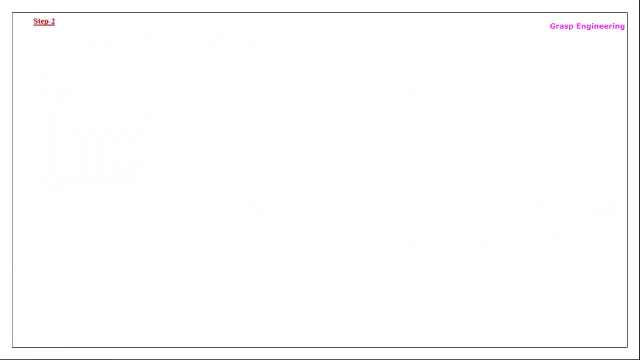 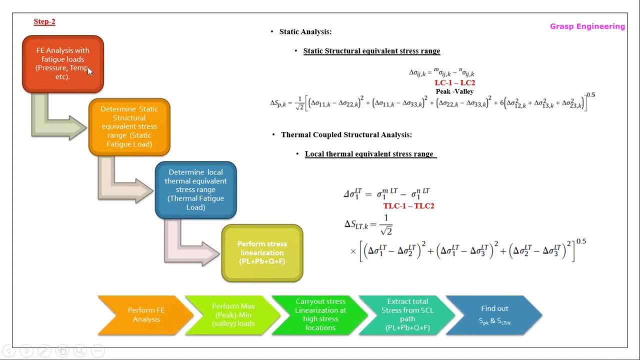 first step. now the second step. as we identified the fatigue loads, then we need to do a fe analysis with the fatigue loads, for example if pressure and temperature case. so once our fe analysis is done, then we need to determine the static structural equivalent stress range. so basically a static. 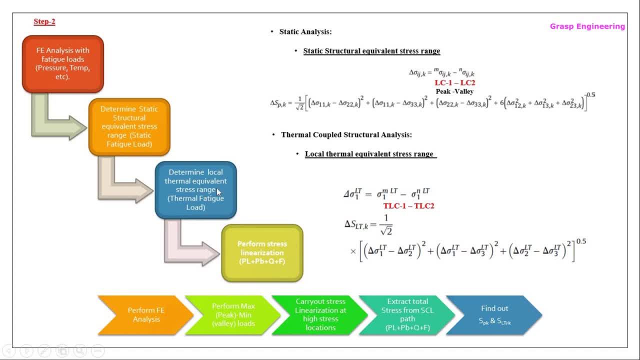 fatigue load and we need to determine a local thermal equivalent stress range. this is basically a thermal fatigue loads. so when we talk about static load, we need to identify a static structural equivalent stress. when we talk about thermal loads, we need to find out the local thermal equivalent stress range. 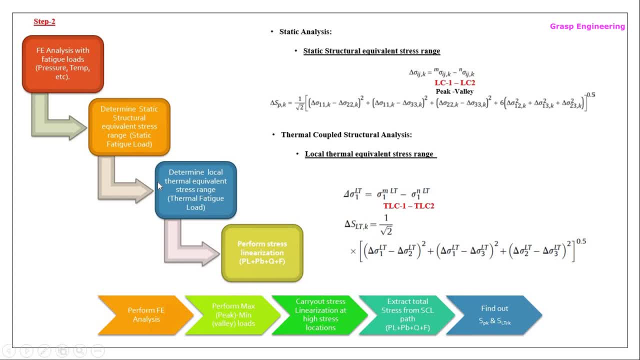 so what does it mean? so if you go and if you refer asm standard, you will find two formulas. so the very first is static structural equivalent stress range. so this can be found out by this, using this equation. so if you see this equation here, it is nothing. 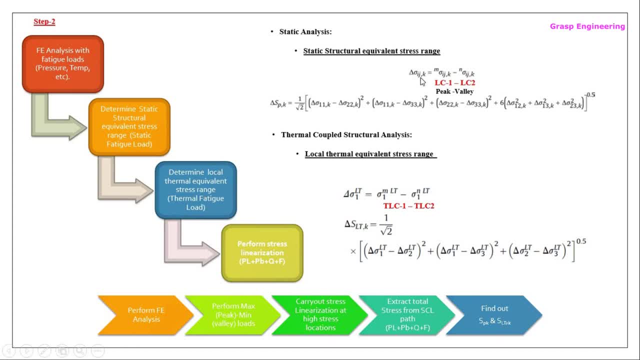 but a static structural equivalent stress delta sigma ijk. and here you, we need to do this from sigma ijk at initial condition minus sigma ijk at the final condition. so basically, load case 1 minus load case 2, that is nothing but your peak minus valley. okay, and this is what your one message. 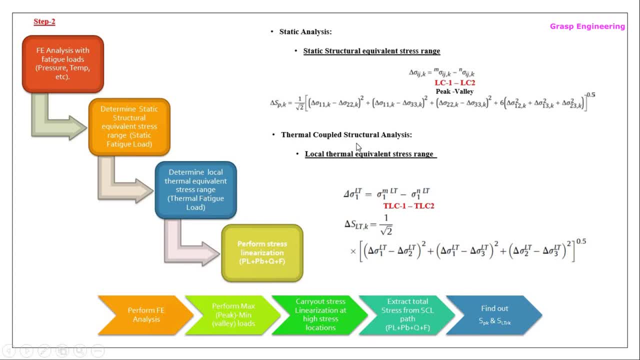 equations. so similarly, we need to do the thermal couple structural and we can easily evaluate the thermal equivalent stress range. so you will find a similar formula over here and here this is thermal load case 1 and thermal load case 2, and once you will identified load case 1 and load case 2, you 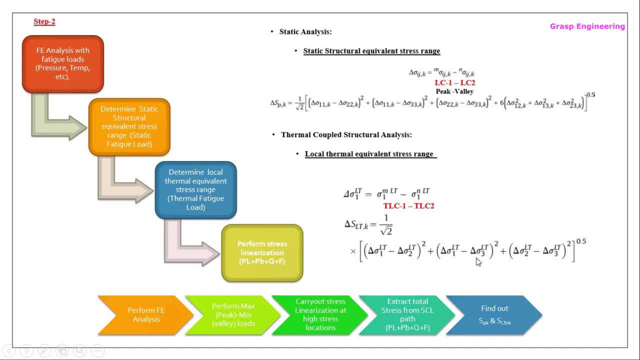 can easily figure out this equation. so these are the two, your equivalent stress equations which are given. so sometimes you will face the confusion. what does it mean? so it is nothing but your one message: stress equations for static as well as static and thermal, hippocampus stress as well as. 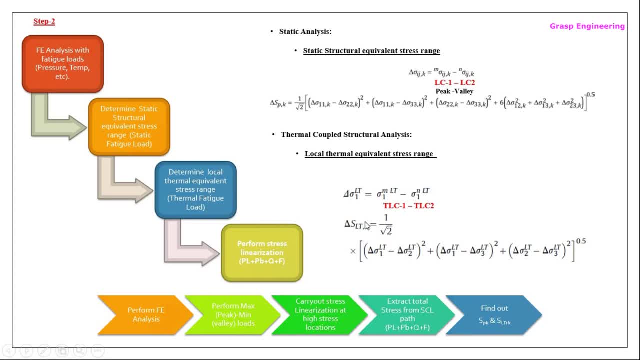 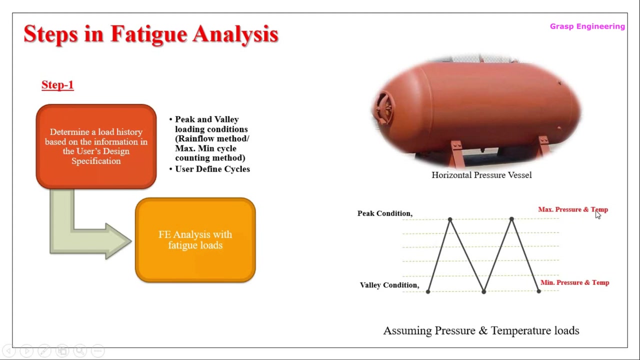 your thermal simulations. so this from there, from this, we will get this delta slt and delta sigma igk. so this delta spk and delta sp ltk. so this value we will going to use in a fatigue equations. okay, so if you see our previous slide here, we know that pressure and temperature when 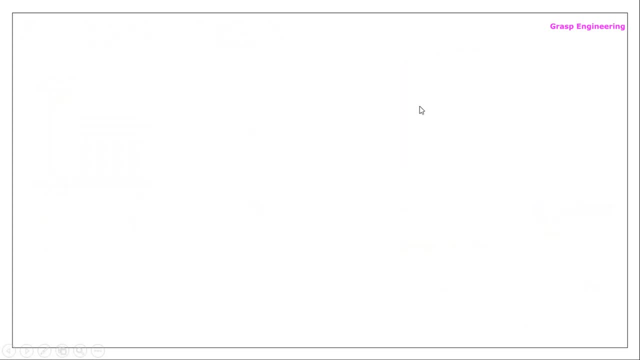 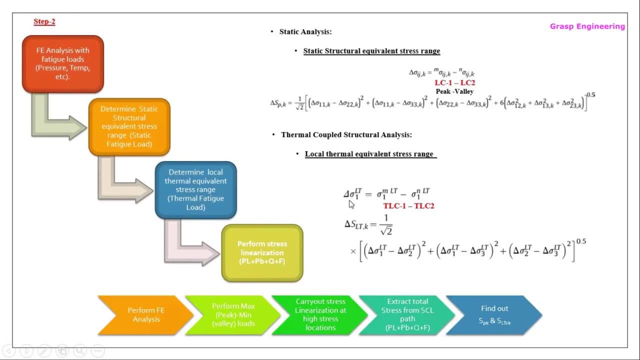 we talk about pressure, minimum pressure and max evasion, we will get delta spk. when we talk about minimum temperature and maximum temperature, we will get delta ltk. so basically it is nothing but local thermal equal stress range. that is delta ltk. so here we need to. 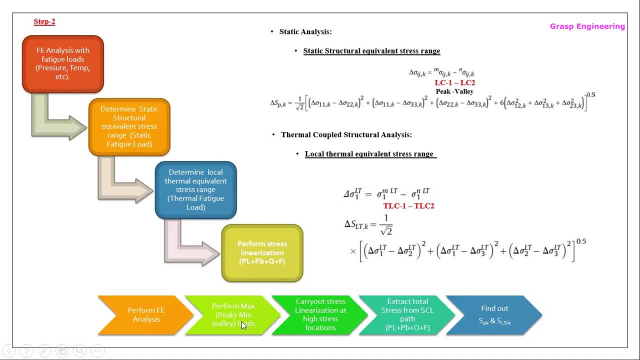 perform epinephrine analysis, perform max and minimum loads, carry out stress relation at high stress local locations and extract the total stress from hcl path, that is, pl plus pb, plus q plus s, and find out the delta spk and delta ltk. so, as we know that these are the one message stress equations, but 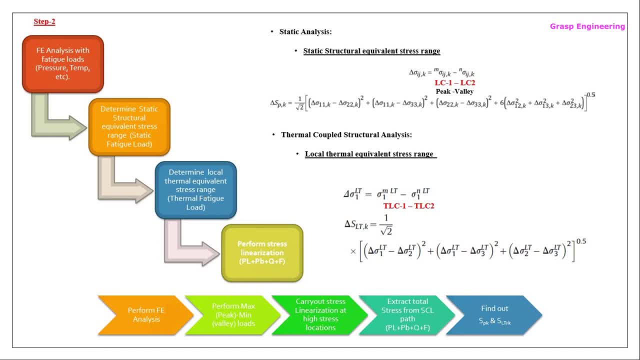 how to extract when we? because if you refer any analysis simulation, you can get the output one message stress equations. so that is basically: if you compare this equation and the output- one message stress equations- you can get the output one message stress equations. and if you see the results given by the fea, both are going to be matched. but here, as we discuss, 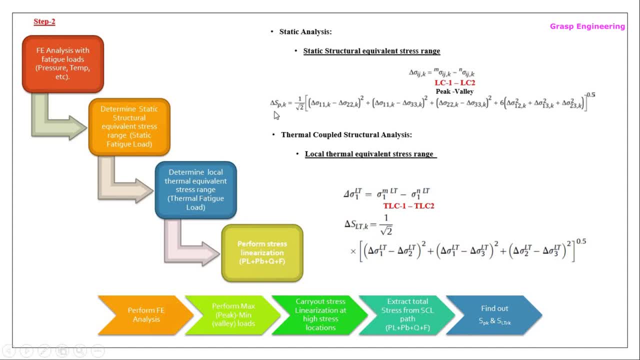 earlier. we need to find out these values, delta spk, as well as delta ltk, through the stress linearization. so here we need to extract the stresses through scl paths at the highest stress locations, and we need to find out pl plus pb plus q plus c l. so summation of all this is nothing but your delta spk. 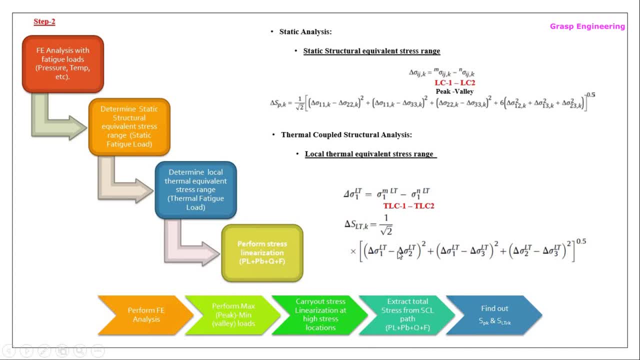 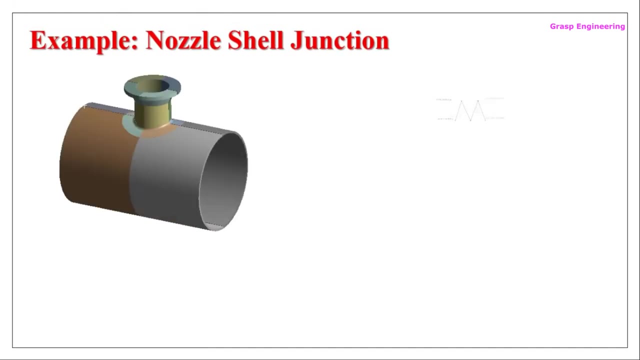 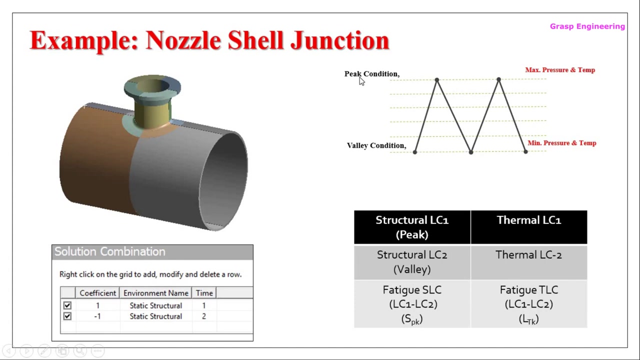 in case of static simulation. summation of this is nothing but delta slt in case of thermal simulations. so we will discuss this through a simple example. so this is one of the example of nozzle shrink junction. consider this nozzle junction and here we will going to assume a 2 load case, that is, peak condition and value condition in case of peak. 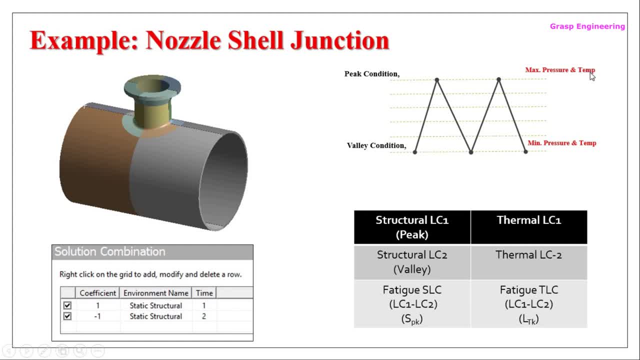 condition, we can consider aCDMlockitation equal to it andllow condition in case if peak condition, a maximum pressure and maximum temperature. in case of valley condition, we can consider a minimum pressure and minimum temperature. so here, as we discuss, these are the structural load case. structural load case 2, that is max. 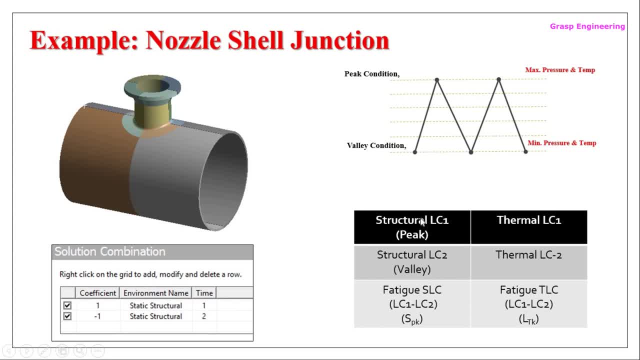 pressure structural load case. sorry, this is structural load. case 1, that is peak, structural load. case 2, that is valley. so this is nothing but your max pressure, minimum pressure and fatigue load case: Delta SVK. how we can figure out that? by my doing subtraction between these two. similarly, we can separate this thermal. 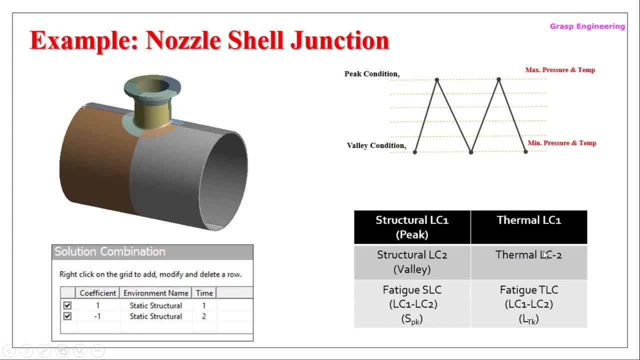 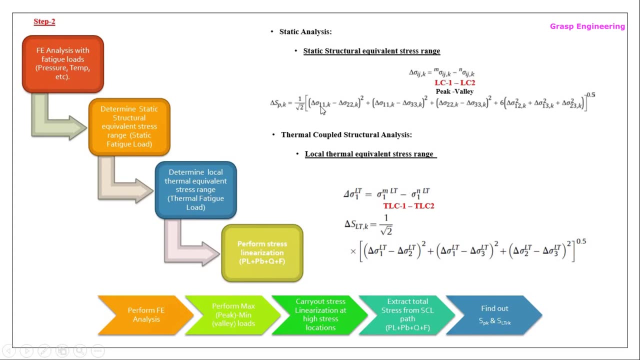 simulation results like max thermal, minimum thermals, and then we can subtract max minus minimum. that is Delta LTK. so if you go to our previous slide, so as we are doing the same thing over here, that is peak minus value and here also you will find peak minus value. so how we will get this? 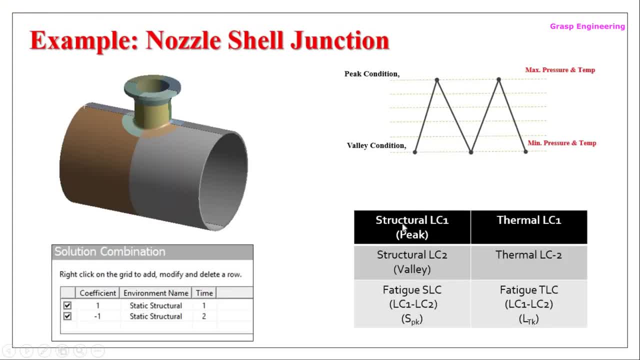 once you will perform the thermal simulation and static simulation, you will get this two value. then you can use a solution combination. suppose, if you have ANSI software with you, then in that case you just use a solution combination and then you can go to your. you can say the tree or you can say the. 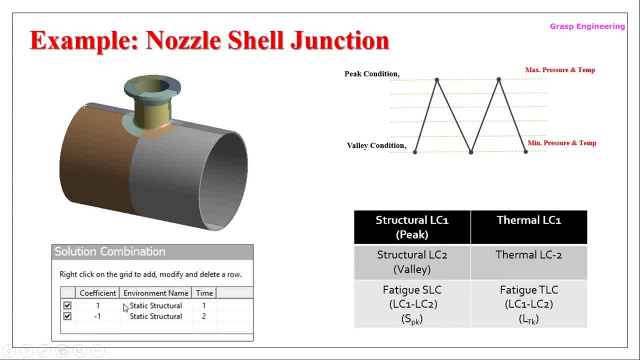 solution combination. if you click on that, you will easily find out this. if you see, this is nothing but your first load case 1 at a time standard 1, and what we are doing? we are keeping minus 1, static, structural and at this, load case 2. so basically what we are doing: load case 1. 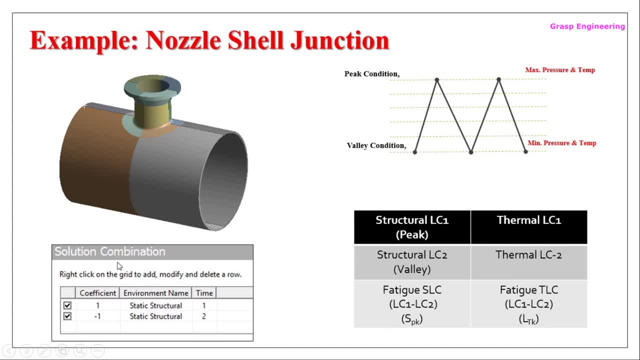 minus load, case 2. so once you will find this solution combination, then you can extract here the results called one message, stress, right, and here at this you can do the stress realization okay, so it is difficult to understand. but once you will go through this, all these steps, then you will get some confidence on this and then you can. 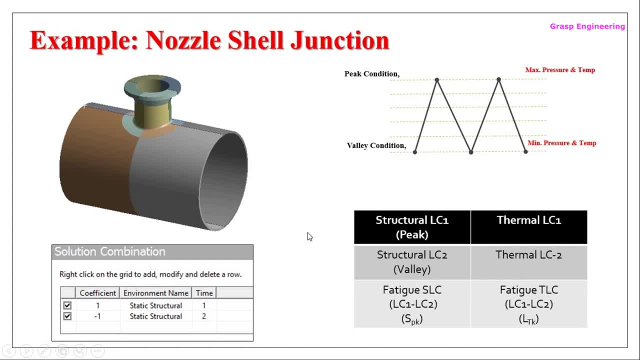 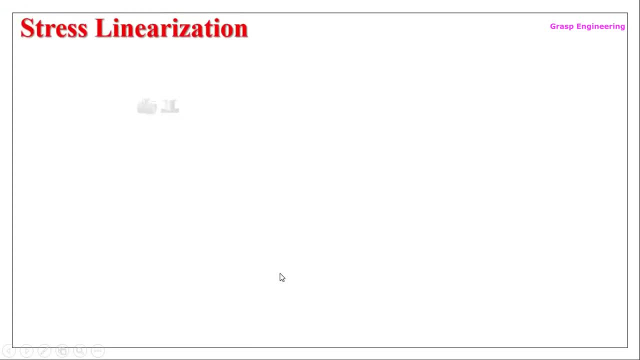 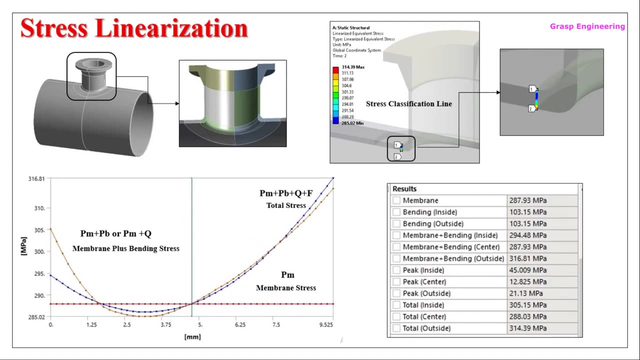 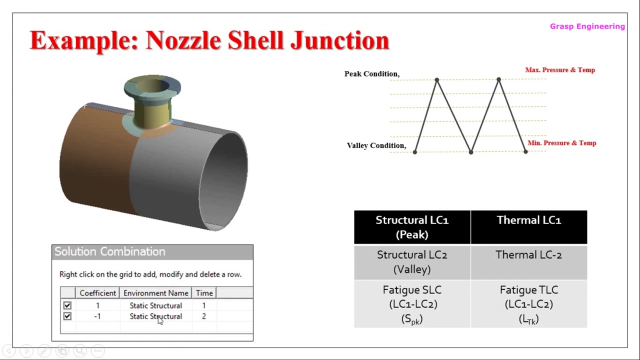 easily figure out how to do this. simulations: okay, we will also discuss the few of the examples now. stress negation: so now this slide represent the stress reaction approach. so if you see, in previous slide we discussed about a solution combination. in the same solution combination you can extract the results like strength variation. now, for example, 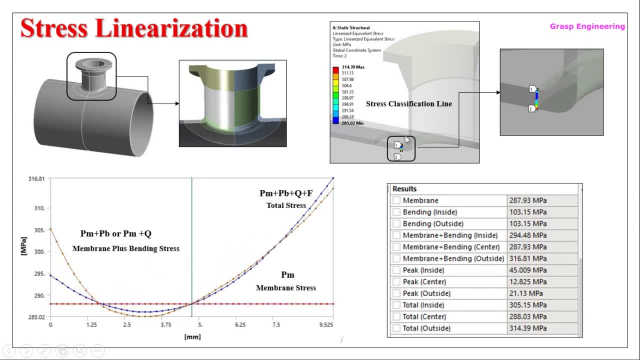 take. we are getting high stress at this junctions. so you just need to do extract this through stress classification line from inside to outside surface. once you will extract this at solution combination, you will get output results like this. so here you will find membrane stress, binding stress, membranes, plus bending peak stress and total stress. so if you 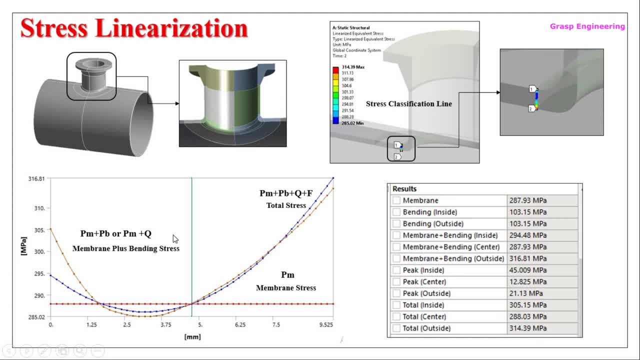 see, this is nothing but your stress base and graph. so here you will find the same result like this is: you are membrane sense, which is constant. you will find over here. then this is what your membrane plus bendy, this is what this line you can find like this and this is the total length you will also 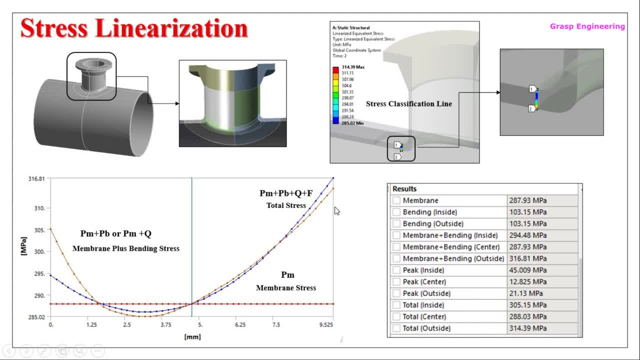 line also here. so basically this pm is nothing but membrane, pb is nothing but bending, q is nothing but secondary and f is nothing but pip. so you will find this total value 314.39 you will find over here. so this value you will going to use as a delta slt right? so this total value is nothing. 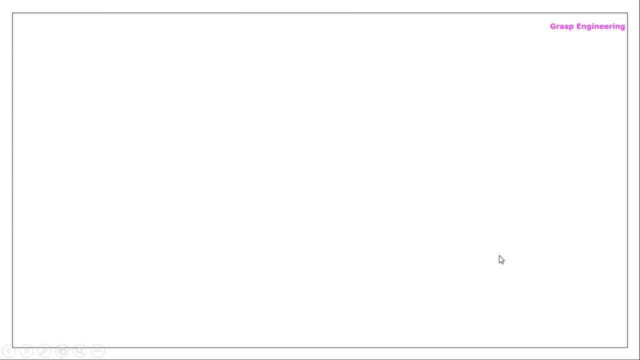 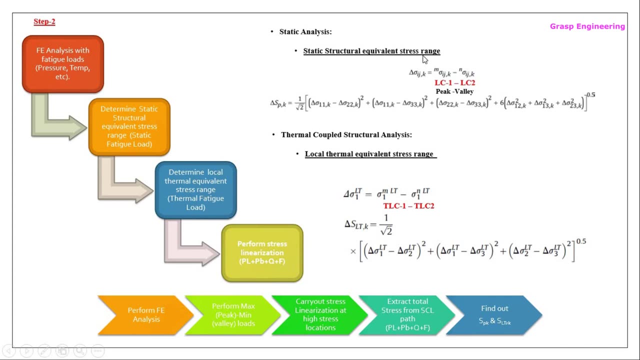 but what? i will go to previous slide further. you can find this: that total value is nothing but your delta spk, that is static structural equivalent stress range in case of static simulation, and that is delta ltk in, that is local thermal equivalent stress range in case of thermal. 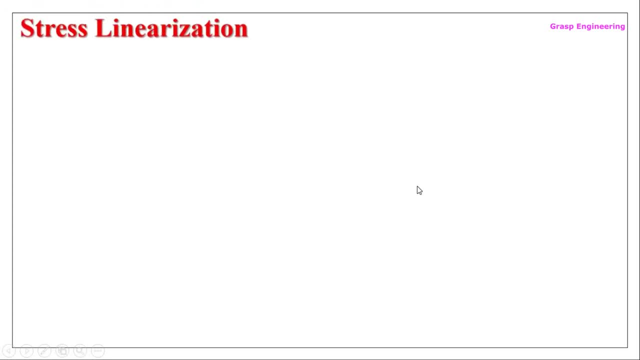 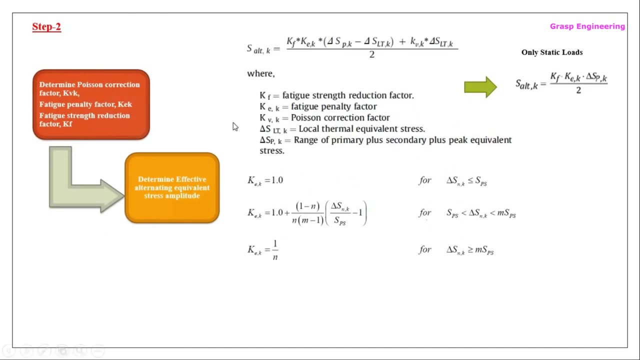 simulation. okay, now we will go to next steps. that is step number three. so here we need to once we figure out delta spk and delta ltk, so you will find this equation. this is nothing but alternative stress equations. so here you will find kf into kek. kf is nothing but fatigue stress reduction factor, kek is nothing but fatigue penalty. 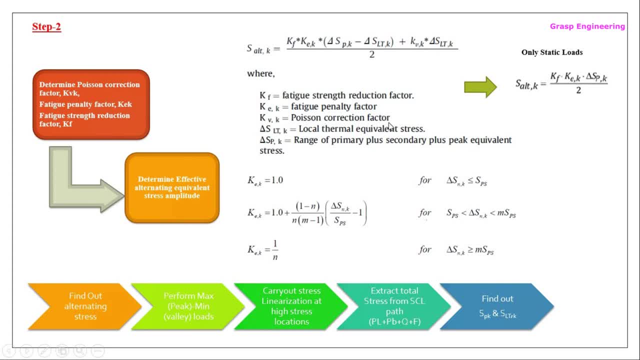 factor and kbk is nothing but poisons correction factor. so these are the three factors we need to incorporate here and here. this is ltk, spk and ltk. this is nothing but local structural equivalent stress range, local thermal equivalent stress range, plus kvk, plus ltk. you just need to put 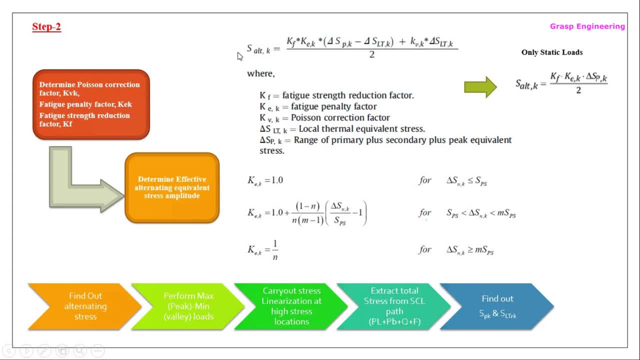 that values in this formula and from this you can easily get the alternating stress and if you refer, these are the fatigue strength reduction factor. these are based on your few factors. you can easily figure out these factors from your asme course and you can just put that values over. 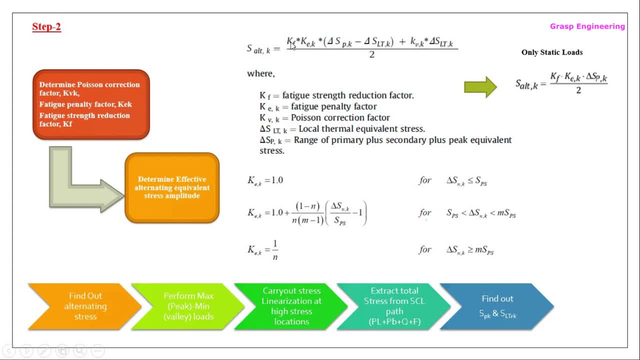 here. if you don't want to go in that depth, you just assume that one and you can easily figure out the alternative stress. okay. so here, if you see, this, k e, k is nothing but one when your alternative stress is less than your sps secondarily primary for secondary stress range. so it is nothing but. 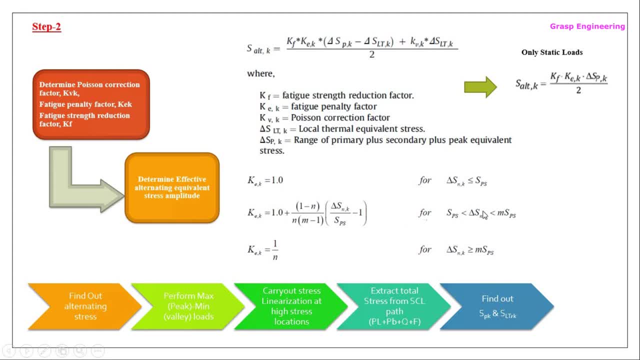 one plus: you need to refer this formula when it is alternating space between your sps and m sps. you need to refer this formula when your alternatives phase is bigger than your m into sps so you can easily figure out: is this an alternative stress for you when the strain 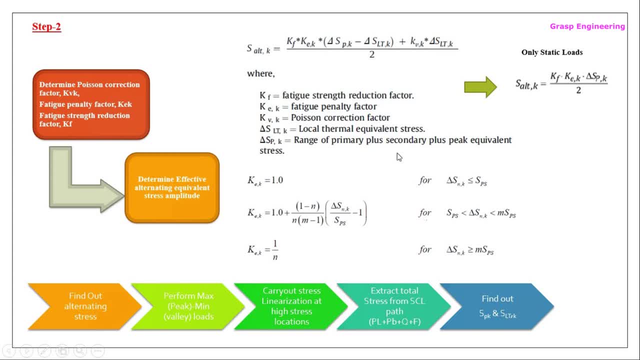 vous avez un intérêt nickname reci reporting technique to understand our sps industry. to bez ayatollah, figure out which values I need to refer for all these three factors. suppose, if you don't have a thermal loads, then your equation, this equation will going to: 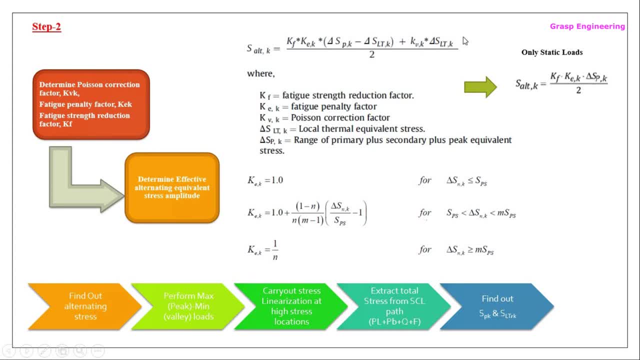 change like this: if you see here this LTK, you can remove and then it will be very simpler: KF KEK into Delta SPK divided by 2. okay, so these we need to determine poisons correction factor, fatigue penalty factor, fatigue strength reduction factor and then we can determine the effective alternative. 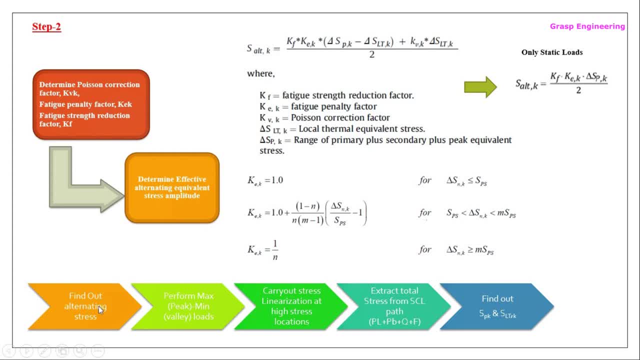 equivalent stress amplitude. that is what this okay. so find out alternative stress. perform max minimum loads- this is the same- carry out stress reagitions path and find out the SPK and LTK. so these are the similar steps, what we discussed earlier. so now we identify our, our alternative stress. 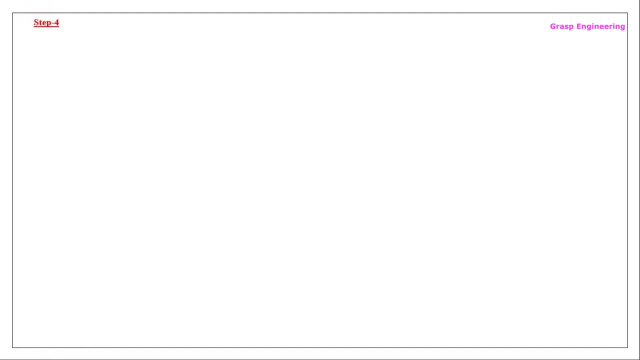 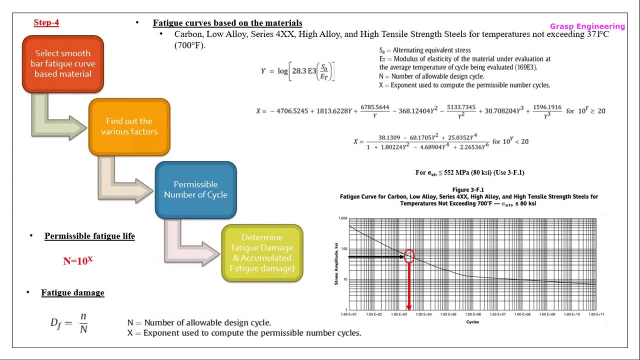 now we can move to our next step, number four. so once we have identified our alternative stress, then what is next? the next step: we need to find out the fatigue curves based on the materials. so here we need to select the smooth bar fatigue curve based on material. so you need to first know what. what are the material configuration or 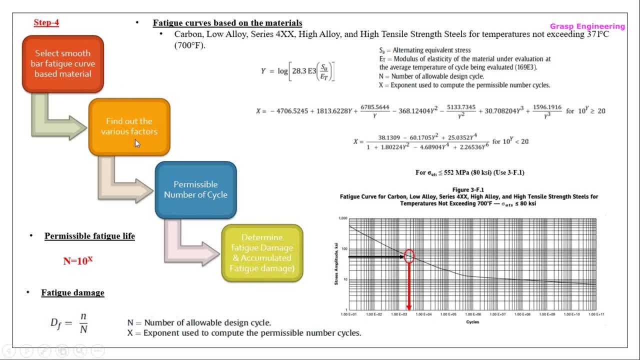 material specification and then find out the various factors based on these equations and then find out the permissible number of cycle and determine the fatigue damage and accumulated fatigue damage. so we'll go step by step. suppose we have a material like carbon: low alloy, series for excess, high alloy and high strength cell. 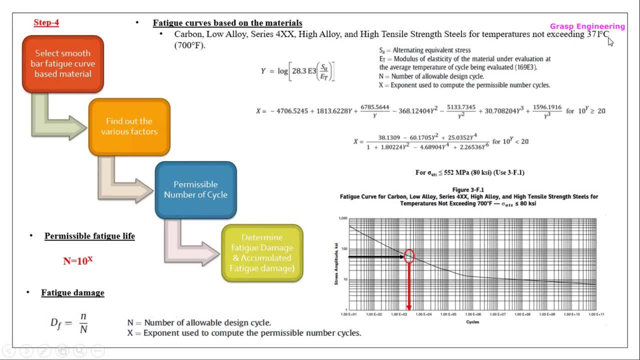 strength steel for temperature not exceeding that 371 degree centigrade, suppose if we have this material. so this is called a fatigue curve 3 f1. then we need to identify the factors. these are the factors X. you just need to refer this formula. you can get this formula from a SME code. you can go to the design. 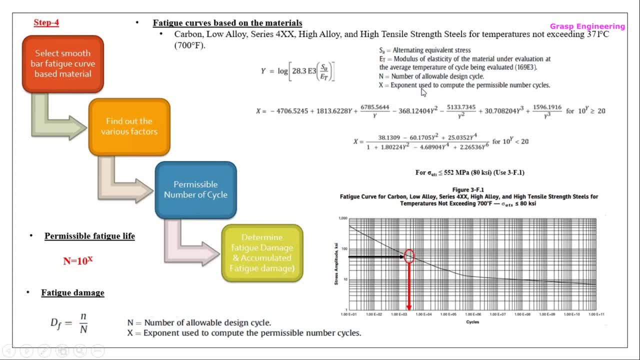 by analysis, fatigue assessment approach. so here this X is nothing but the exponent used to compute that permissible for a number of cycle. so these factors are based on your this material data curve, so you can easily get this factor when you refer this respective clause. okay, so from this we 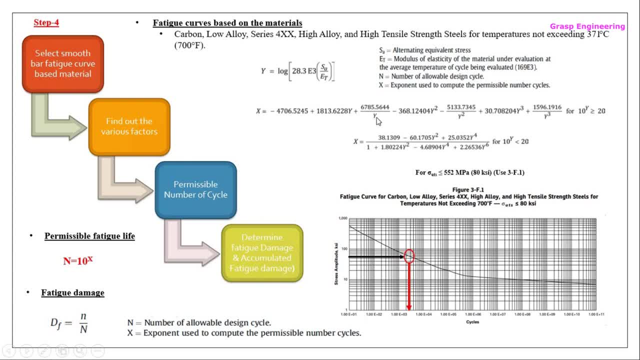 will get the X value, the very first we need to identify the Y. Y is nothing but log of 280.3 E3 into SA. SA is nothing but equivalent stress. what we find in previous step, that alternative stress, is nothing but equal to E3. E3 is nothing but equivalent stress. what we 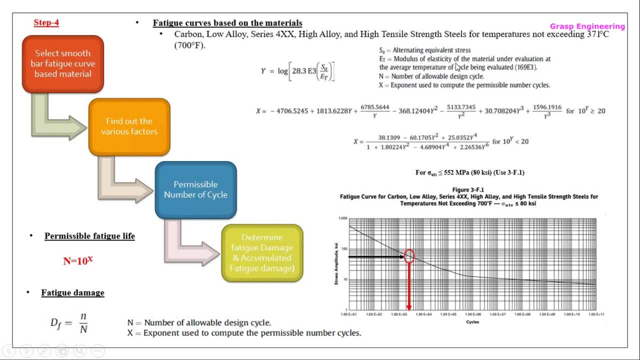 find previous step that alternative stress is nothing but equivalent stress, saying we need to put over here and it is nothing but modulus of elasticity of the material. so once you will put SA and ET value, then we can get the Y value. then this Y value we can put over here and we can easily identify the X value. 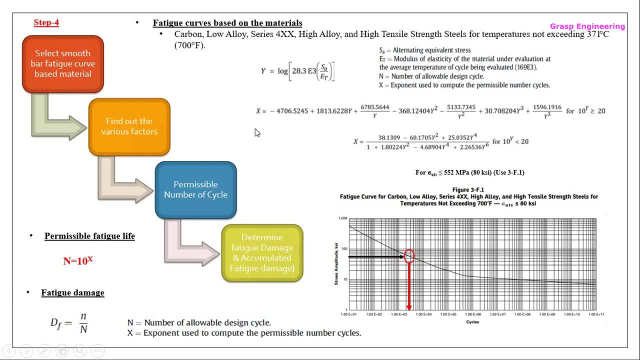 so if you see, once you will identify the X value, you can easily get the permissible fatigue like cycle. that is nothing but N is equal to 10, raise to X. so if you see, we assume this material and for this material, if your alternative stress less than 552 megapascal, that is 80 ksi, if you have this much criteria, then we can. 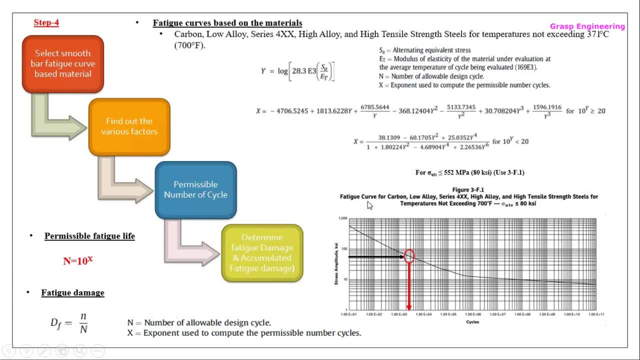 use this 3f1 and this is what the one of the graph for fatigue curve 3f1 for the same material. here you can easily identified your alternative strength. so suppose, if your alternative strength is nothing but between this 10 to 100, so you just drop a line, horizontal line this, find out this point and draw a. 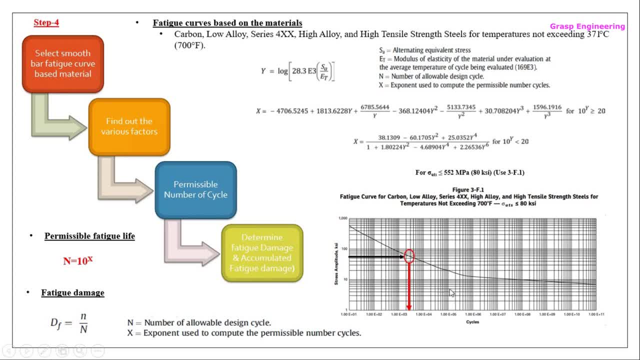 vertical line, then you can easily identify the number of cycles. this is, through the graph, the similar fashion you can do with this equations, okay. so once you will find the permissible number of cycles, then you can easily find out the fatigue damage. so fatigue damage is nothing but the ratio of. 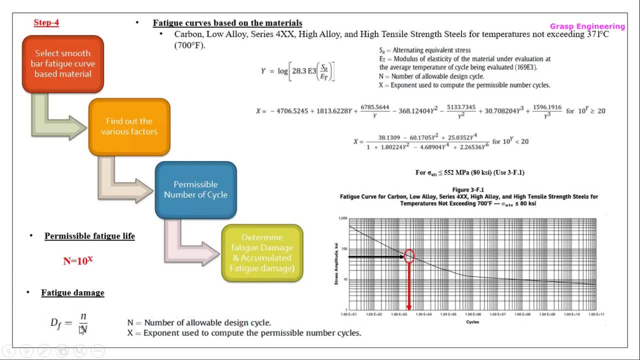 number of allowable design cycles per unit, your permissible number of cycles. so for that you should know your permissible number of cycles. suppose, designs, suppose I am getting a 300 cycles from this permissible fatigue cycles and I am having the 400, you can say the 400- design cycles. so this: 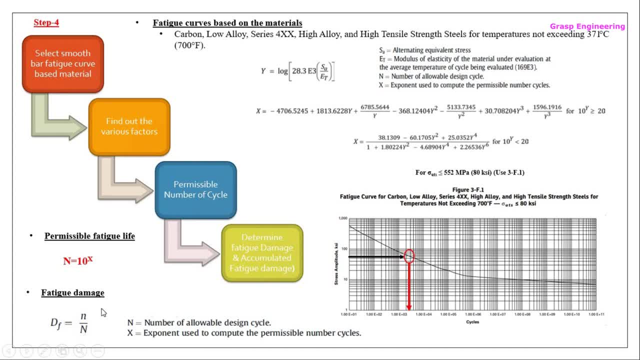 design cycle 300 by design 400. so you can easily find out the fatigue damage. it should be always less than 1, then you can say you have a more number of of, or you can say the more number of cycles than the design cycles. okay, so always keep in mind your. 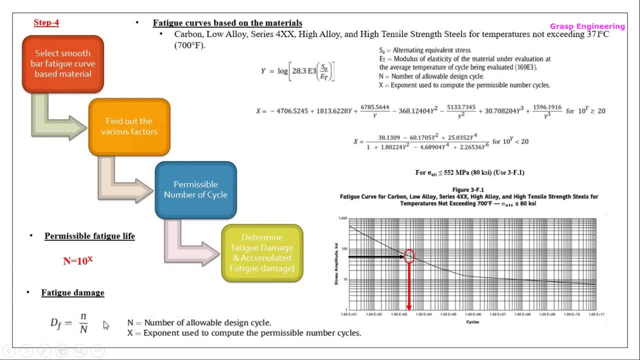 this time. so i think we can. i will explain this further here. what we did we? first, in previous slide we just identified the sa alternative strain. then we need to find out the permissible cycles. with this equation that is nothing but n is equal to 10 raised to x. so here x we can find out. 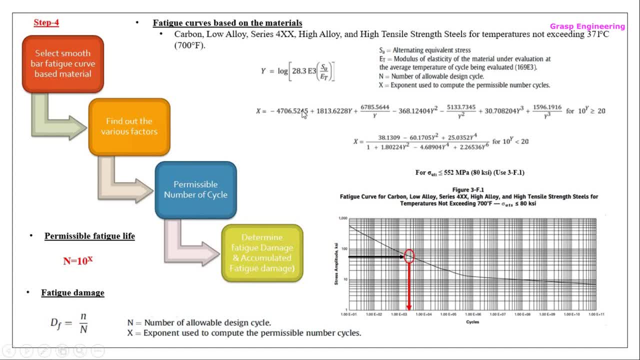 why this formula? and for this formula, you will find these are the different factors which we selected based on our material definitions. and here we will find this y. so why we find out by this formula that is, y is nothing but log of 280, 3, e3, sa by 80. and here we 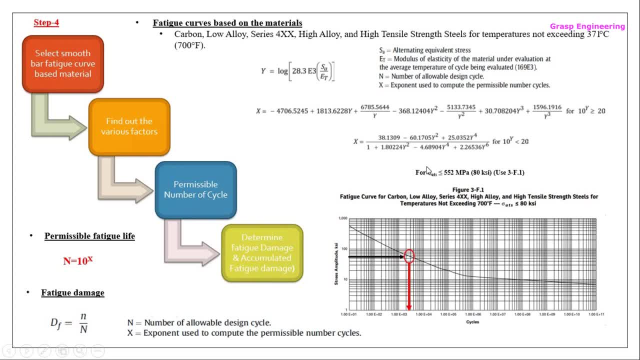 can put our alternative strain. so these are the different steps which we need to follow you, if you refer your asme code, you will find a lot of difficulties, but if you refer this video, you can easily figure out the how to find out the permissible fatigue cycles and fatigue damage. 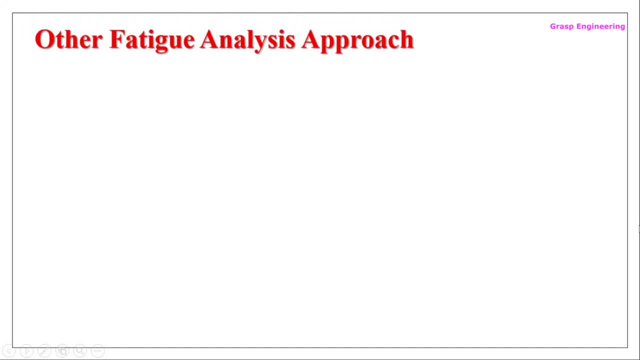 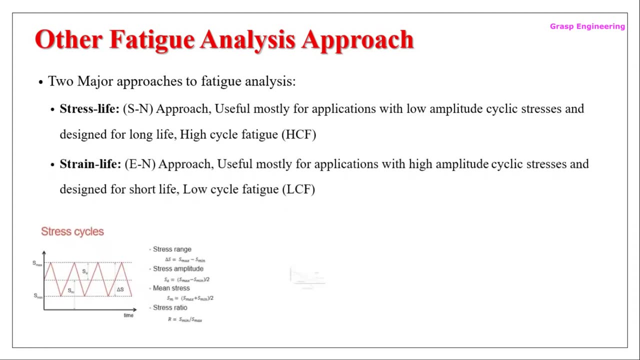 so this slide represents other fatigue analysis approaches. earlier we discussed about asme based fatigue analysis approach. now there are two major approaches which are widely used to perform a fatigue for asme and asme based fatigue analysis approach. so this slide represents other fatigue analysis approaches. earlier we discussed about hope- single type fatigue change and portraying that. 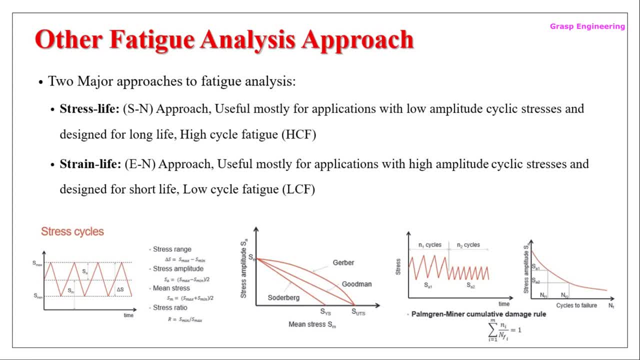 sadece unnecessary fatigue67. so as an approach. the second approach is like strain light approach. here you will find e? n approach. it is useful mostly for application with high amplitude cycle is called aztres life approach. so we see the first is a stress life approach. so we see high cycle fatigue life analysis approach. how do we find this in washington university? 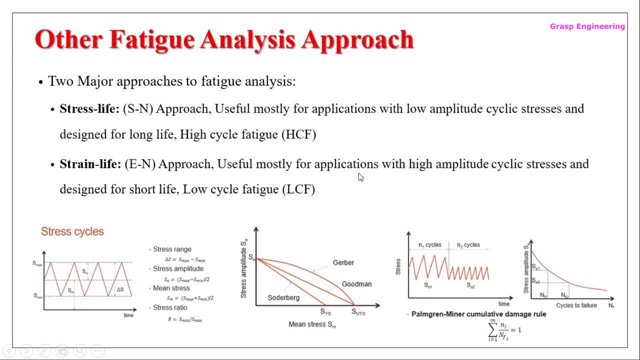 see how you find this in is england university EN approach. it is useful mostly for application with high amplitude cyclic stresses and designed for a short life low cycle fatigue. So both are the opposites when we talk about high cycle and low cycle fatigue. Here we need to do the same. 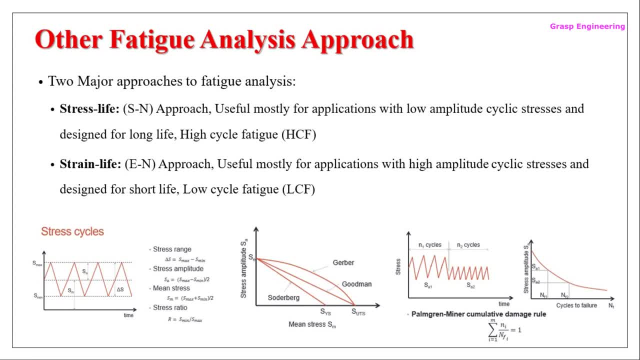 We need to carry out the FE analysis and then we need to find out the principal stresses. And, if you see the way, very first we need to find out the stress cycles. Here you will find like for stress range, That is max minus, minimum, So basically value minus your peak conditions, and then we need to find out the stress amplitude. 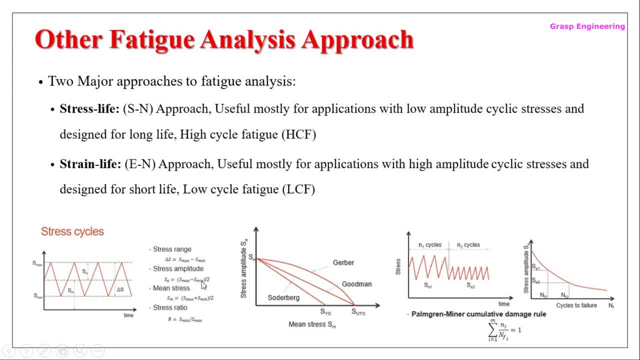 that is nothing but your alternative. stress X max minus X minimum divided by 2 and Later on, we need to find out the mean stress. So for both the approaches we need to find out mean stress. So here we need to do the mean stress corrections as we studied, you might have studied in our academic 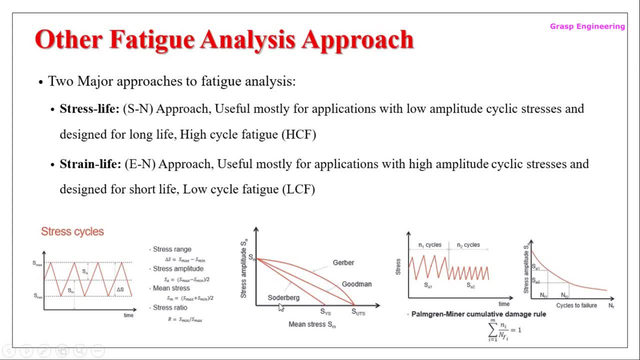 for a Like. we need to do a mean stress correction either by Soderbergh, Goodman or Gerber diagram. Okay, once your mean stress is corrected, then this can be used to find out this stress ratio. Okay, and this you will find. this is what the minor cumulative damage rule. so, in order to find out the fatigue damage, 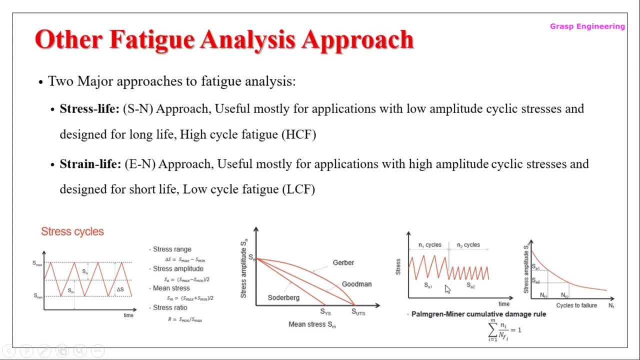 So here you will find the first cycle and it is also accommodating the another cycle. So there are two duty cycles are present and for that, these two duty cycles, If you refer this graph, this is nothing but your stress versus cycle or failure, permissible number of your, you can say, the life. 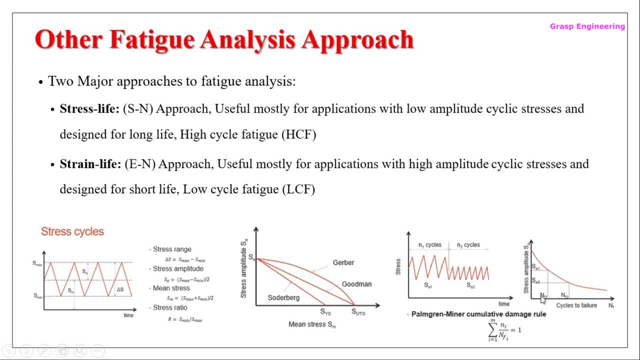 the for first stress, you will find the life. For the second stress value, you will find the another life. So all this cumulative effect can be calculated and then, finally, the fatigue damage is calculated. So that is done by this minor rule. So, similarly, if you have more number of cycles, you can easily accommodate that and you can find out a cumulative fatigue damage. 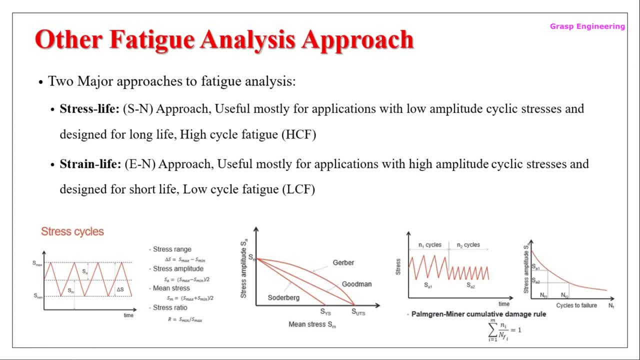 In order to find out the permissible life cycle. So these are the two major approaches which are used. then the question come into mind why we are not doing mean stress correction in case of ASME based fatigue, Because, if you see, We had a refer, some fatigue curve. So this, all this fatigue curves already. 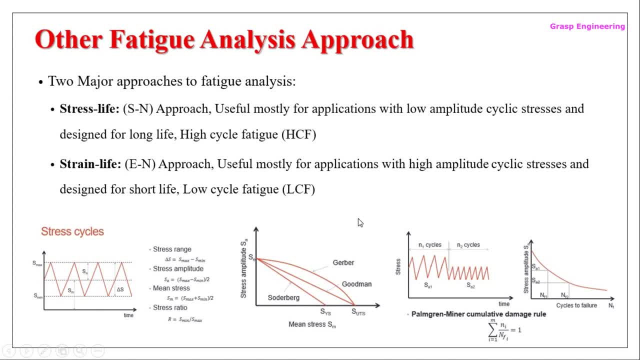 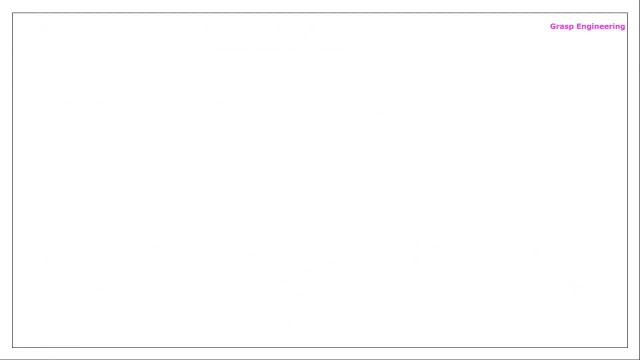 Tested with the mean stress corrections. So that's why there is no mean stress corrections. when we talk about ASME fatigue analysis approaches Now we will discuss about the few fatigue analysis examples. So, like we will discuss the three examples of fatigue analysis based on ASME approaches, 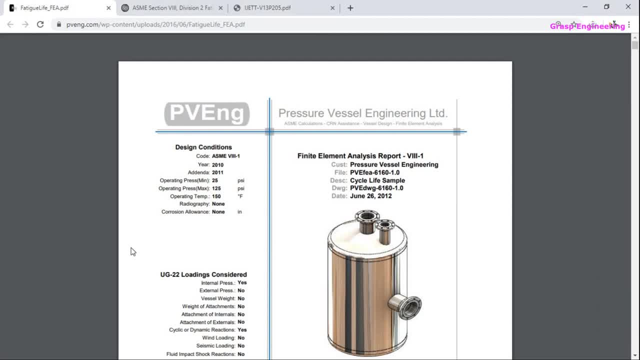 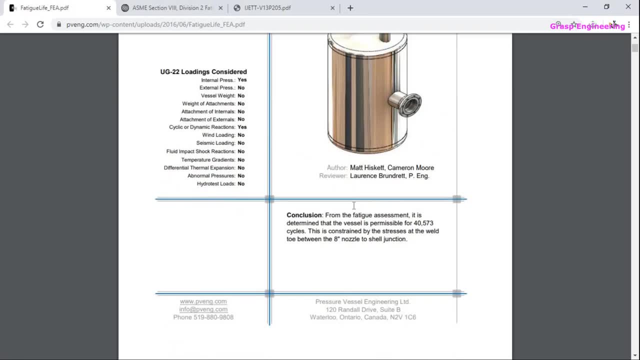 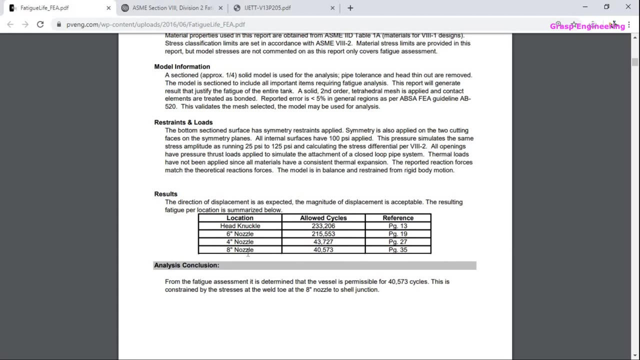 So now we will discuss the very first example of You can go to pressure vessel engineering, limited PV engineering. there You will find the one of the fatigue analysis report. you will find this is one of the vertical vessel and Will go at it down. it may consist of your nozzle. three nozzles are there. 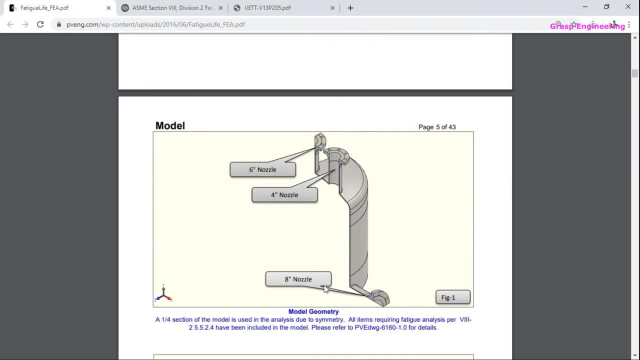 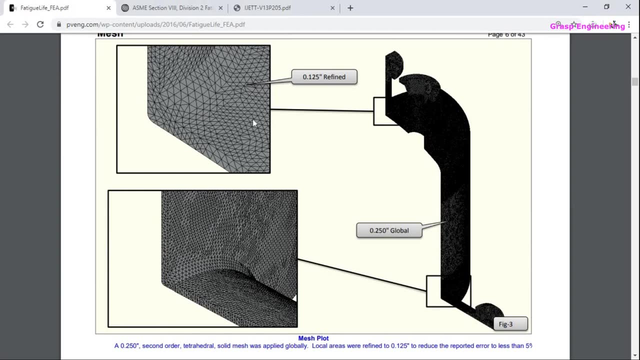 So you will find this is six inch nozzle, four inch nozzle and eight inch nozzle and They did meshing. This is a second-order tetra mesh Or might be a first-order tetra mesh. They did more refinement over here. You will find 0.25 here and more refinement here. That is half of this, and 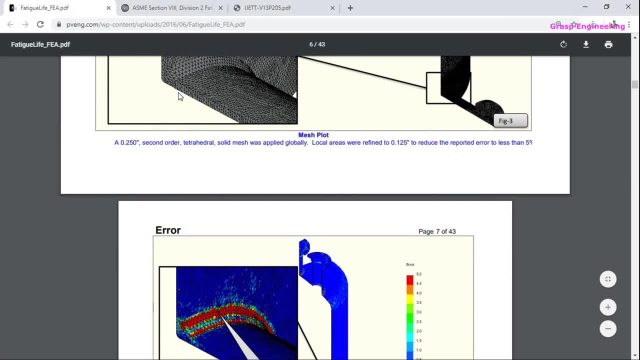 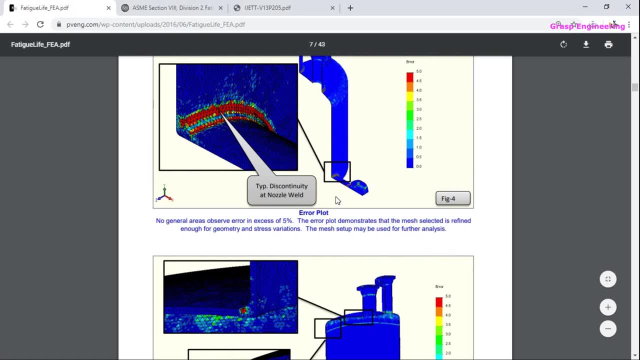 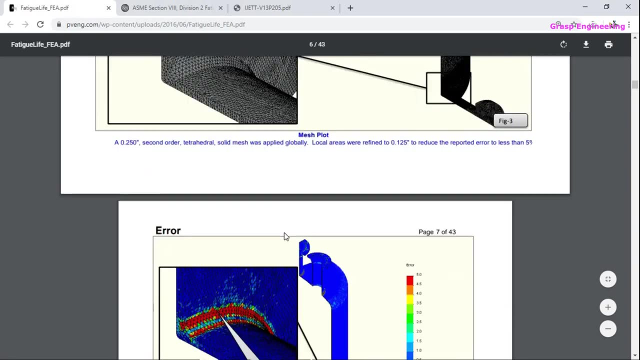 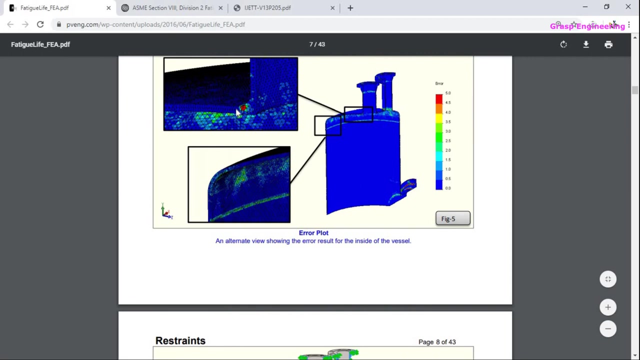 There are two elements. what we saw, Two elements across the thicknesses, and they further did the mesh sensitivity study, So they will find some more refinement over here. if you have a mappable geometry like this, then I will suggest to go with hex dominant mesh and always keep minimum three elements across the thickness. 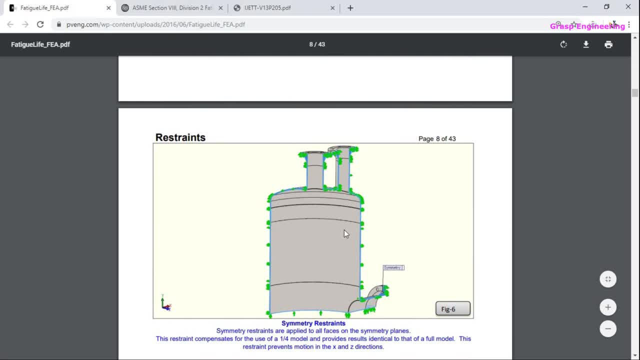 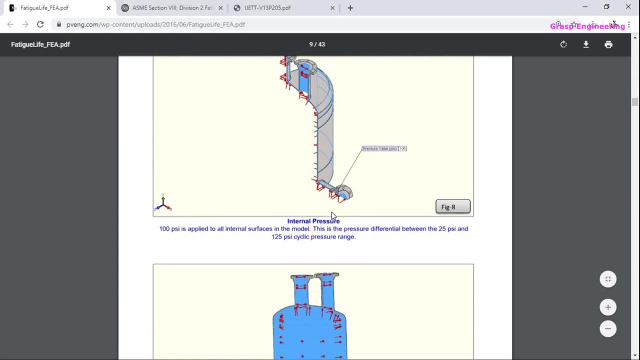 Two elements are not that much sufficient. They use the quarter symmetry. You can find the symmetry boundary conditions Here. also you will find the pressure value application. now They applied an internal pressure, so you will find 100 psi is applied, all internal phases and 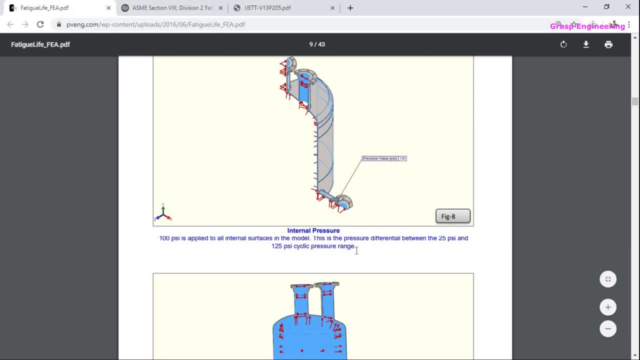 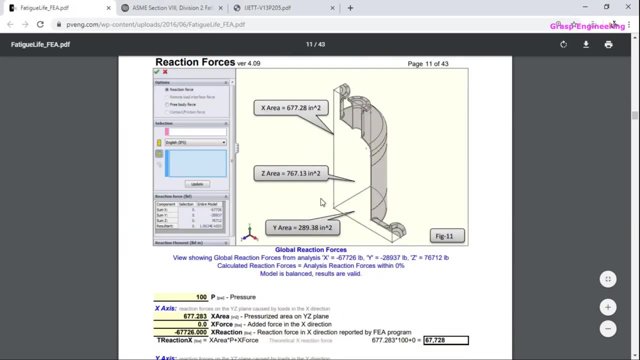 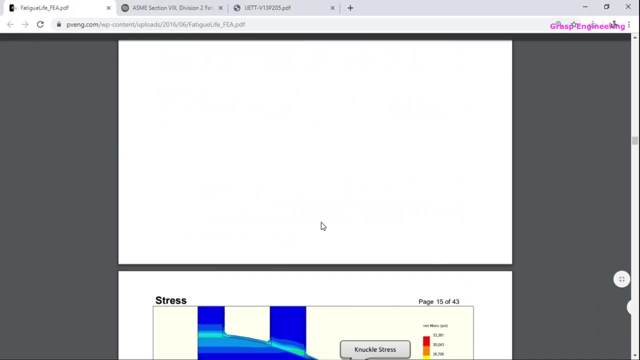 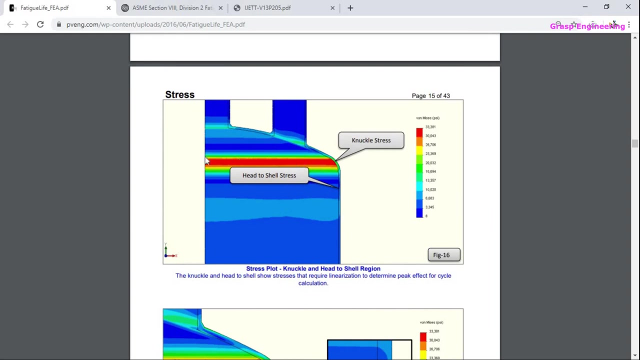 This is the pressure differential between 20 psi to 125 psi. So minimum and maximum pressure values are defined Right. Then you will find these are the displacement value for the internal pressure And we will go to quickly the assessment part. now, if you see here, This is what your stresses, stress cause, one message: stress part: You will have maximum stress at the knuckle region and 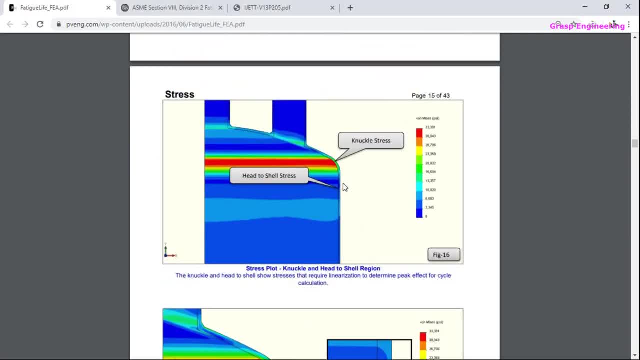 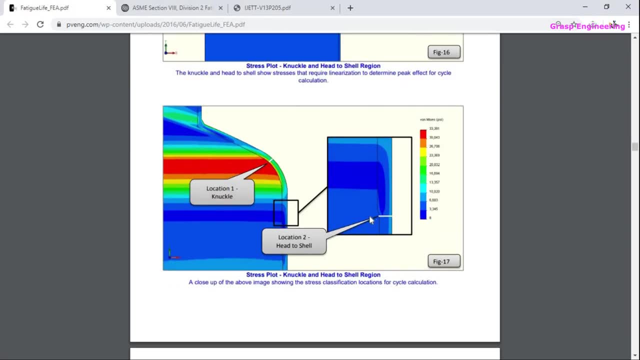 You will find. this is one of the locations where we need to do a stress realization. So they identified the two Location. one is at the junction, or you can say at the knuckle region and at Another you will find at this head and shell junction. So these are the two locations which they identified and 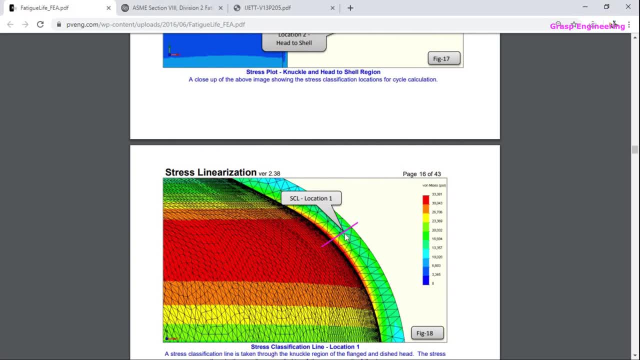 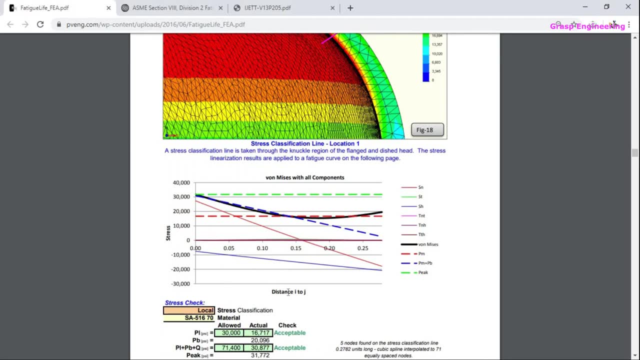 You will find you need to extract a stress relation path like this at various risk stress locations. So once you will extract the path, you will find the output like distance versus stress. and these are the different Graphs, or you can see the different lines which are indicating your. one message: stresses your membrane, stress membrane plus bending. 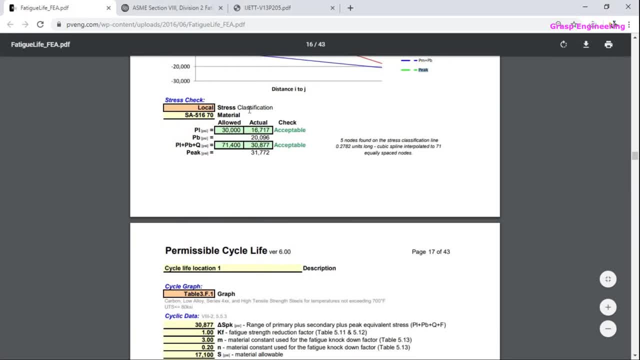 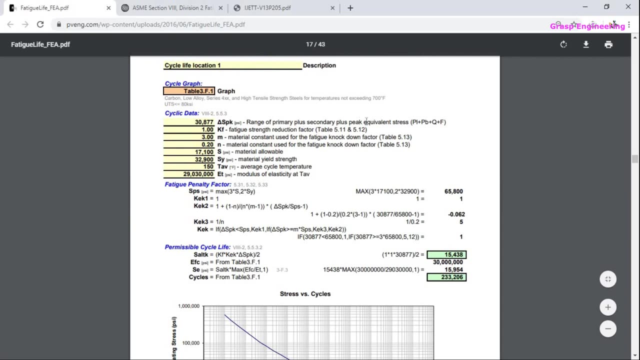 and peak stress. okay, and you will find here the values which are reported, like: what is pi, what is pb, membrane stress, bending trace, membrane plus bending stress and then peak stress. okay, so from this we can easily calculate the delta spk, that is, range of primary plus secondary plus. 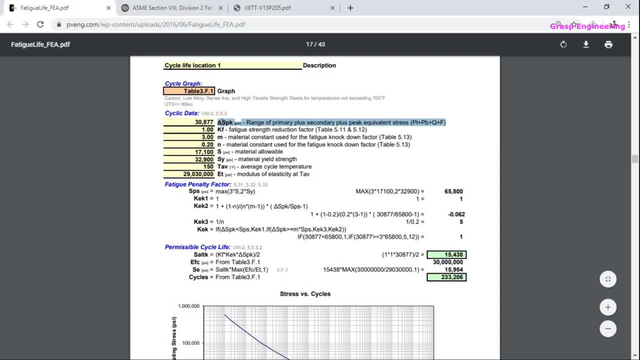 peak equivalent stress, what we discussed earlier. and then we need to identify these factors, that is, fatigue strength reduction factor that we need to refer from the table material constants and this is what that formula, uh, this, this is what our alternating stress formula k of kek into delta spk. delta spk is nothing but what we find out from stress realization. 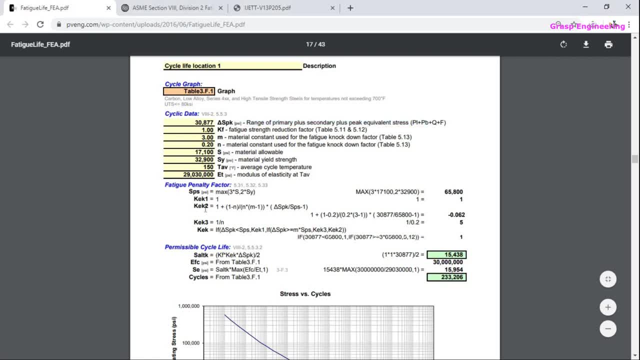 and then these are the different factors: KEK is 1, KEK is 2. these are the three. if it is your less than alterating strengths, then you can use one. there are different things, what we discussed earlier. so accordingly, you need to select a proper value of KEK. then you. 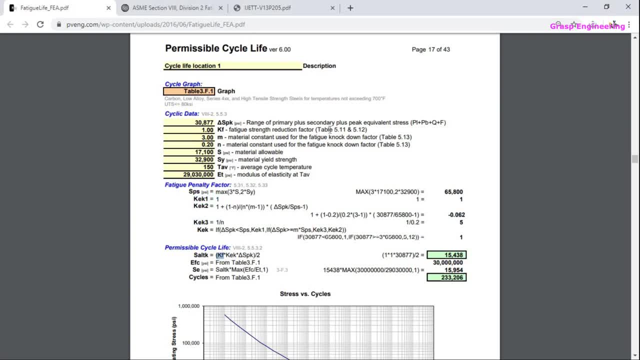 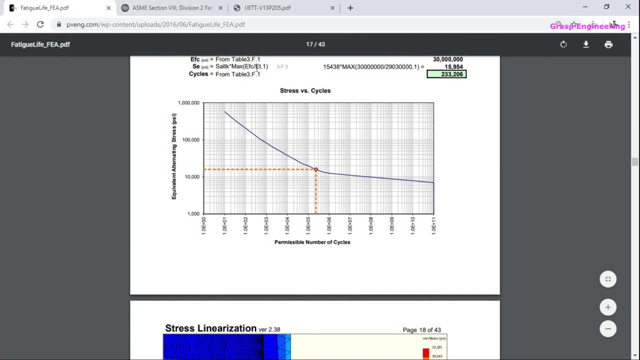 can also add KF fatigue strength reduction factor from the table based on your weld quality. okay, once you will put all the factor, you can easily identify the alternative stress and then later on you can find out the SE, that is, S alternative max of EFC by ET. okay, once you will get your SE, then you. 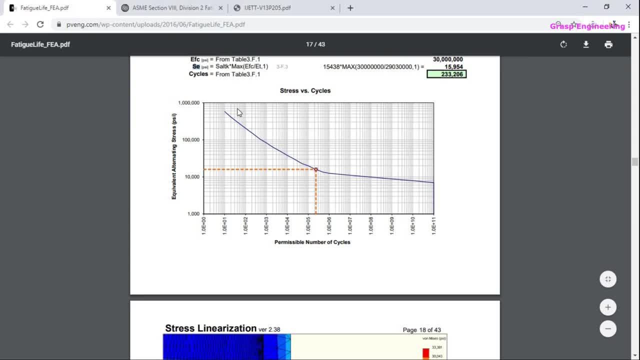 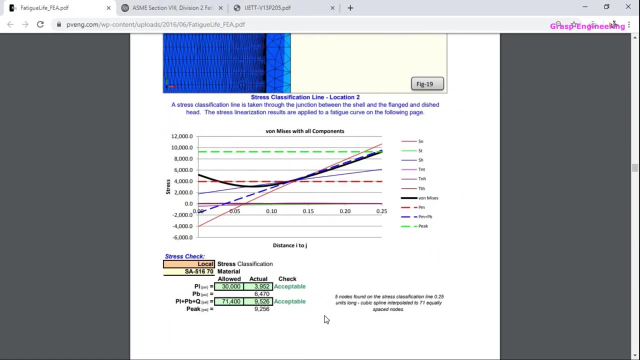 can easily figure out. just put the refer, the respective graph based on material details, and just easily identified the your permissible number of cycles. or you can go with the approach, what we discussed earlier, analytical approach. okay, the same thing you need to follow. for the same thing you need to follow for the same thing you need to follow for. 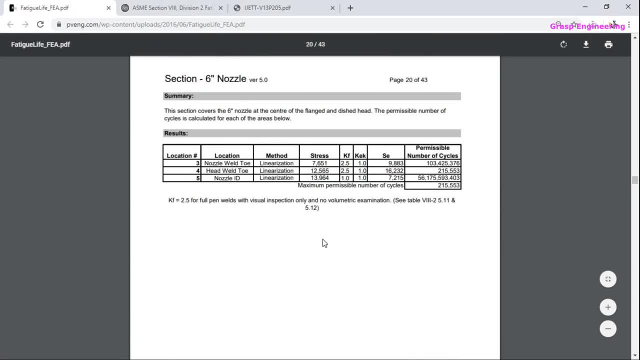 other locations and, at last, you just need to see what is the permissible number of cycles. so they identified at three location: nozzle weld, toe, head weld toe and nozzle ID, and you will find the different permissible cycles for each every locations. okay, so now we will discuss the another problem. now you will 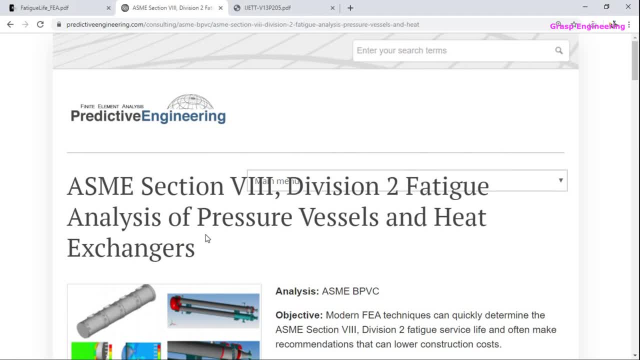 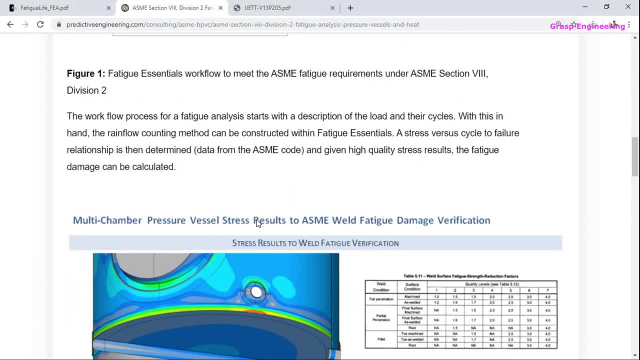 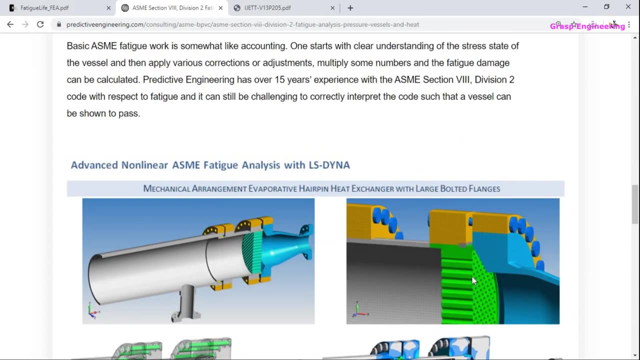 also go to predictive engineering. that is a semi section. 8, division 2: fatigue analysis of pressure vessel and heat exchangers. this is one of the rough summary will go to last. so at last you will see this is what your heat exchanger. this is the tube sheet and you will find the high. 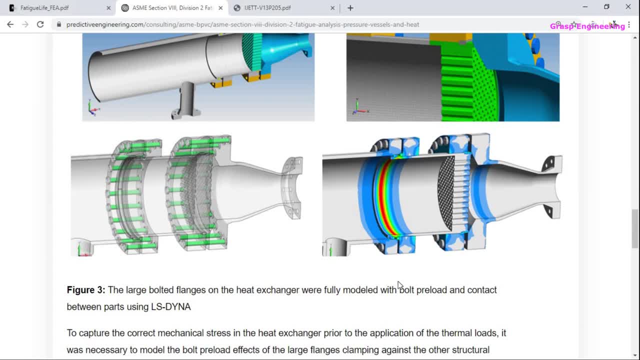 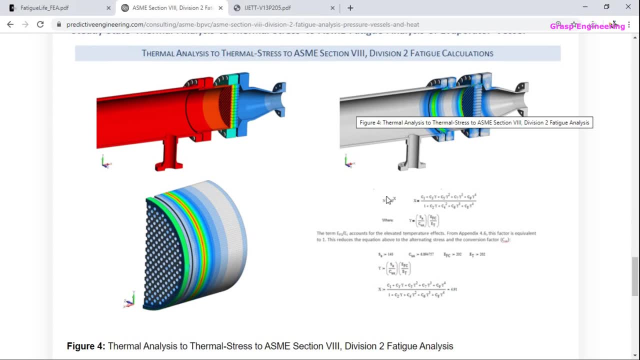 stresses at this location, which is identified the red color. so, and if you go to last, they did the similar simulations. they first calculated the alternative stress and they find out the n is equal to 10 raised to X. so, similar approach. you need to follow what we discussed earlier in order to do the fatigue. 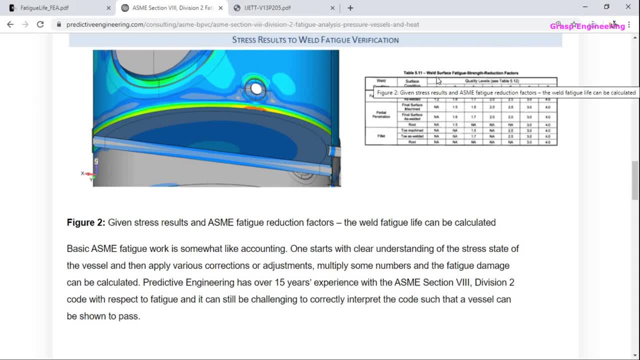 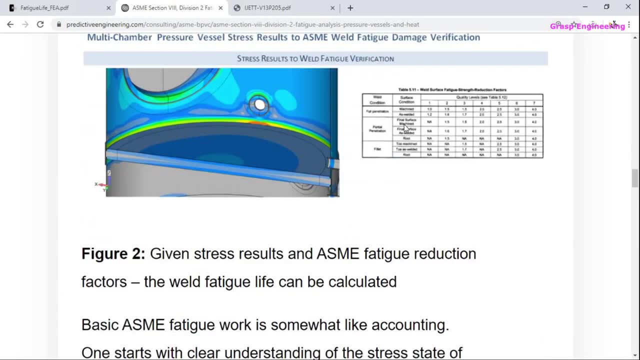 simulations here. this is what the summary for weld surface fatigue strength reduction factors. so it is basically selected based on. if you refer asma, you will find a table like this. so, whether your weld is full penetration, partial penetration or fillet weld, and also based on your surface quality, you can see there are seven quality levels: one, two, three. 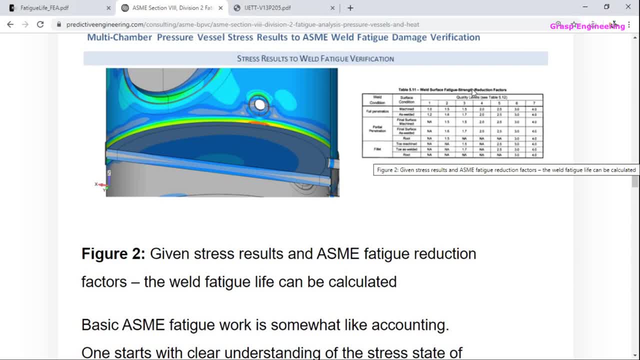 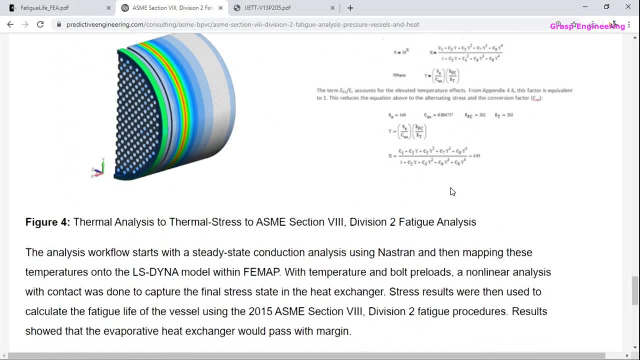 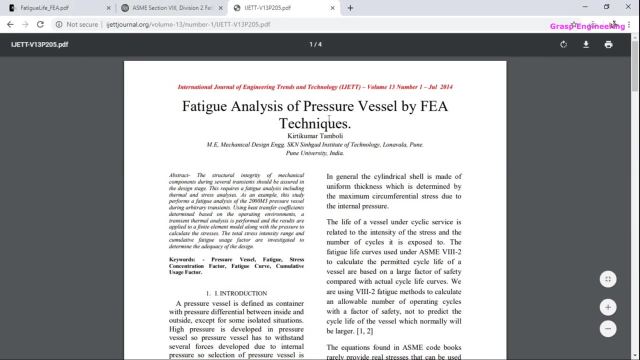 four. so from that you can easily identify what is the value of your fatigue strain reduction, and then you can put that value and your formula and then you can identify the alternative stress. okay, so now we can discuss the next example, that is so your fatigue analysis of pressure. 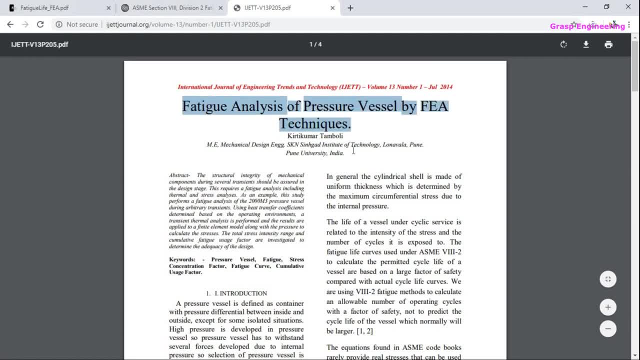 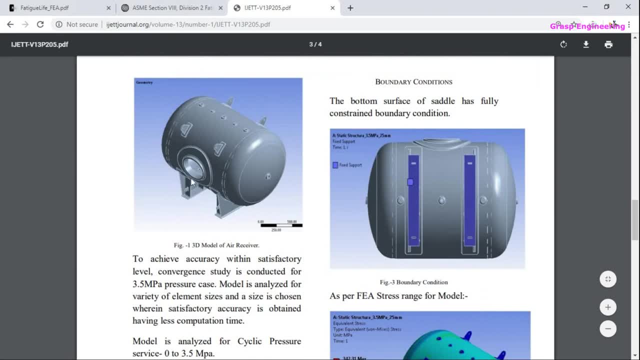 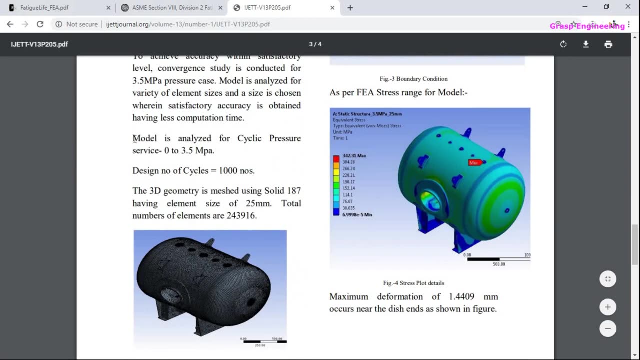 vessel by if a technique. this is one of the paper published in international general of engineering, trades and technology. now i will quickly go to here you will find this is horizontal pressure vessel. it is supported at the bottom you can see the saddle support and here the model is analyzed for a cyclic pressure service. so here zero is minimum pressure. 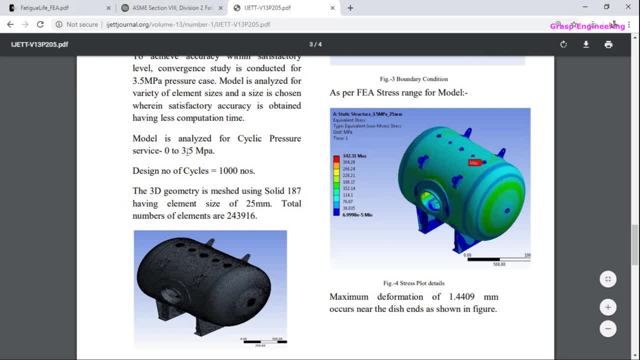 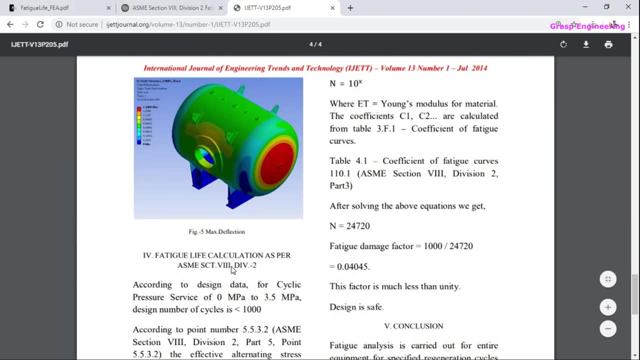 and 3.5 is maximum pressure. so basically valley and peak conditions are defined and the permissible uh. also the design cycles, are 1000 numbers. they use solid 187 element, so basically the tetra mesh they had used to capture the geometry and later on they find out the alternative stress. if you see, this is what your alternate uh equivalent. 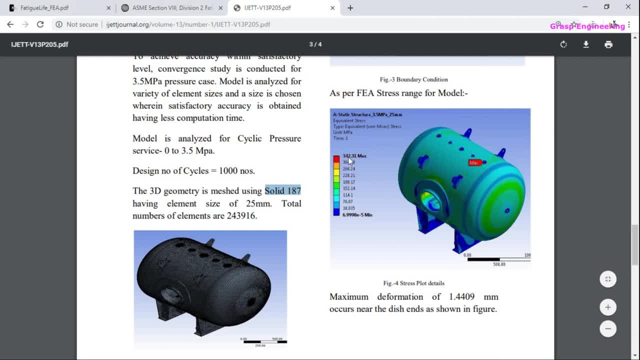 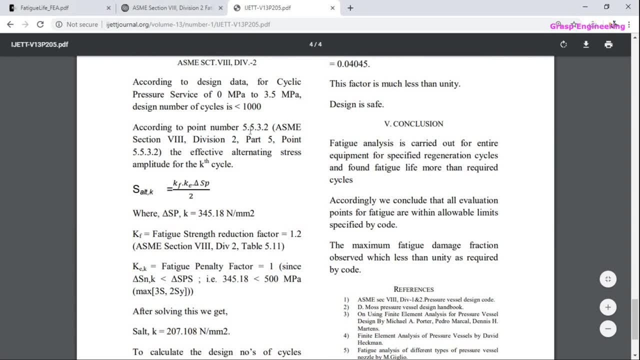 stress, maximum stress they are finding here 340 make 2 megapascals and you will see the similar approach they followed according to 5.5.3, what we discussed. they find out the alternative stress, so k of k, delta, sp, delta sp. what we got from uh stress realization, or some of the uh, if you see some. 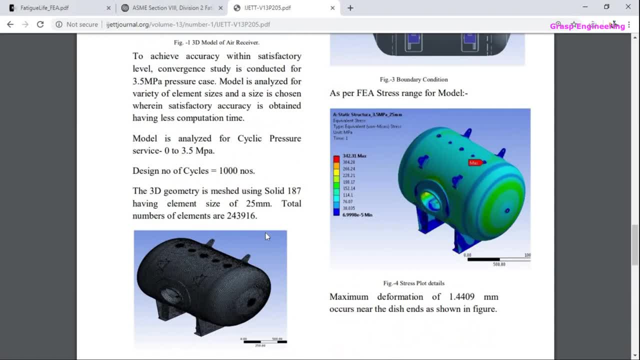 of the stress you can say. the analyst also refer most of the times these peak values instead of doing stress relations. they can easily identify where i am getting this value. if it is at the critical location, if it is excluding stress concentration, then they can even use these values. 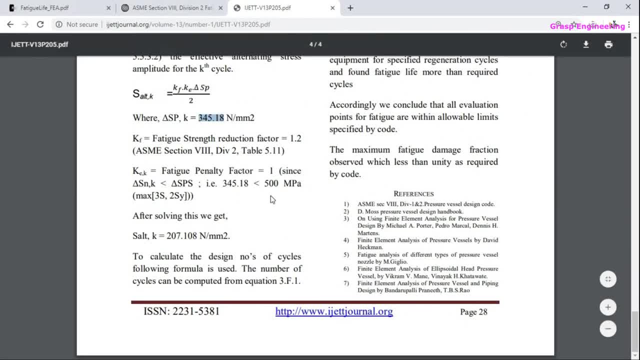 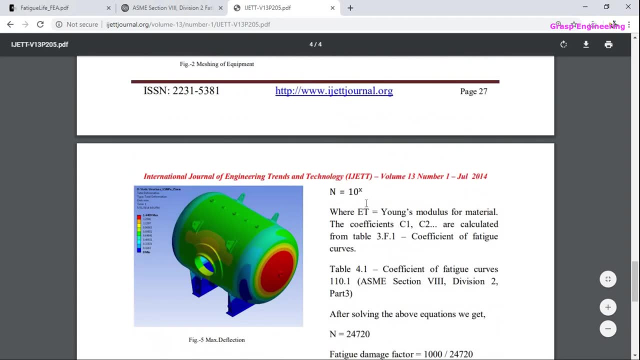 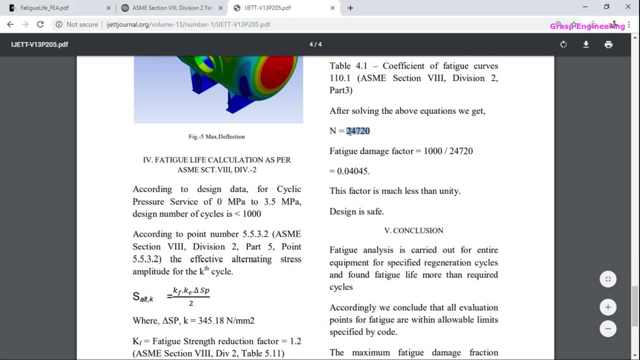 so, similarly, here also you will find he use the same values. okay, then you can put this value over here and you can calculate the k of n, k, fatigue penalty factor, and you can easily identify the alternative stress. okay, once your alternative stress is identified, then you can use this formula and here you can uh easily identify this life as we know.